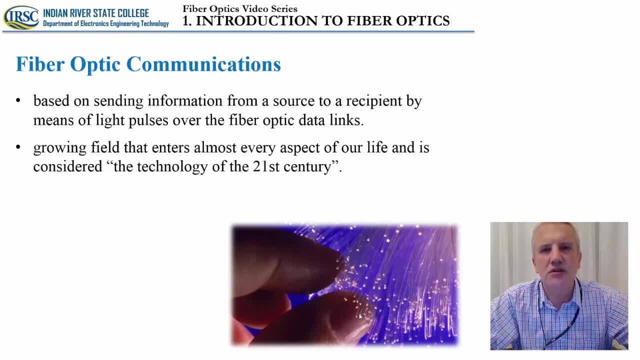 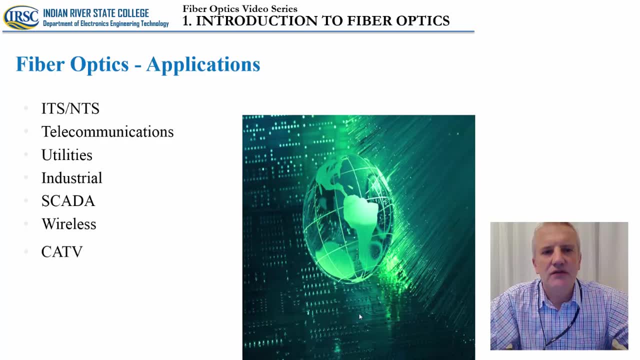 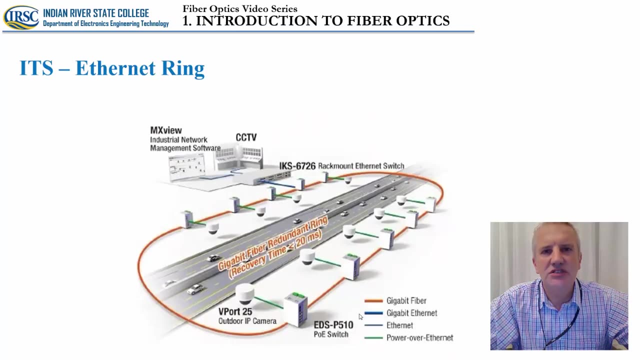 this course and many other courses and training in which you can learn more about fiber optics. There are many different applications out there where the fiber optics has found its place, from telecommunications utilities, industrial systems, SCADA, wireless, medical applications. Let's just 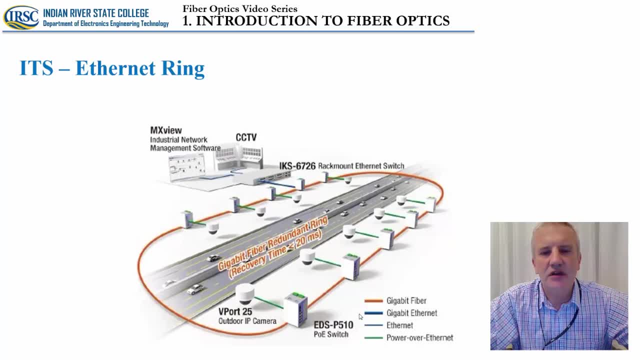 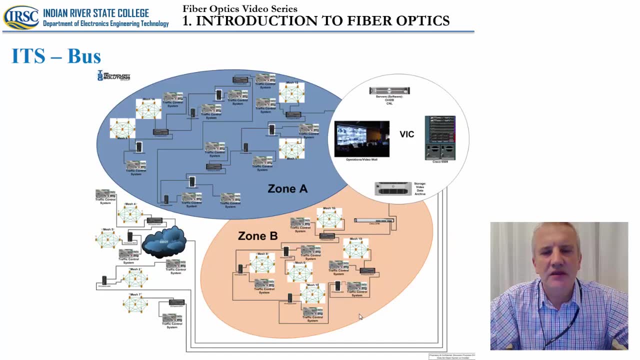 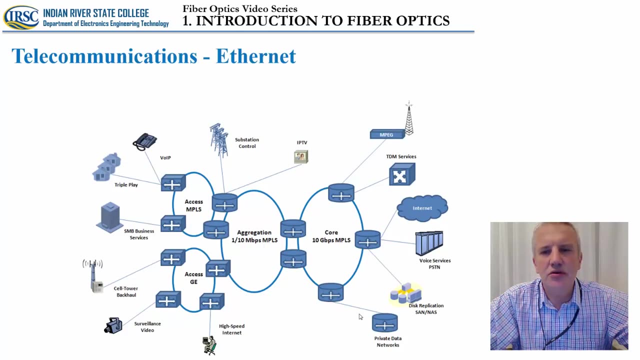 mention a few Here. we have an example of an ethernet ring where different video cameras in the city have been connected using optical fibers. Here's a bus configuration of a specific network. Then we have ethernet that connects many different end users and many different devices. Certain networks are also applied in the industry We are dealing here. 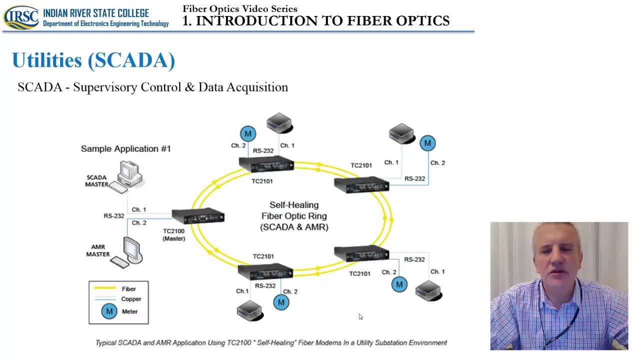 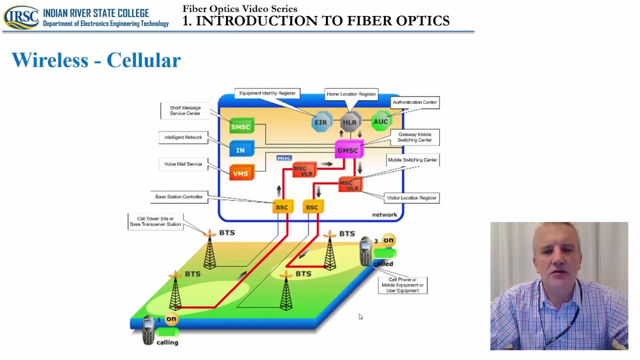 with industrial internet. There's also SCADA systems, where optical fibers are being used for supervisory, control and data acquisition In wireless communication. wireless towers are connected using optical fibers. Here we have a few most recent applications, such as fiber to the home. 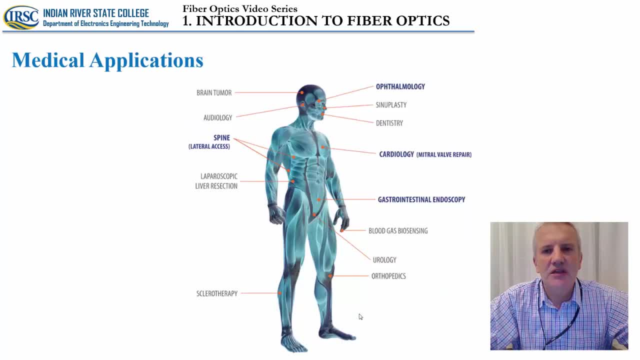 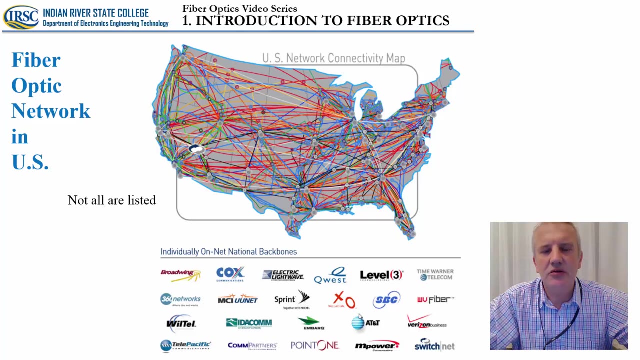 fiber to the building and more generic FTTX, And then, finally, we also have the medical applications, So you can see a very broad range of applications where optical fibers are being utilized. This slide represents the fiber optic network in the United States. You can see many different fiber optic links that are connecting 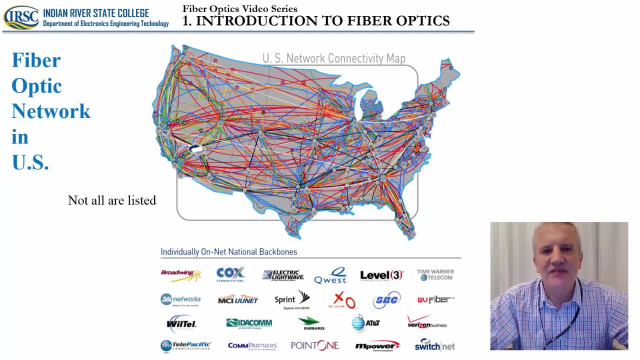 regionally, from the west coast to the east coast. Fiber optic links are also now established in regional local communities. Just recently, many local communities are establishing fiber optic network that connects the end users and the end users. So this is a very broad range of applications. 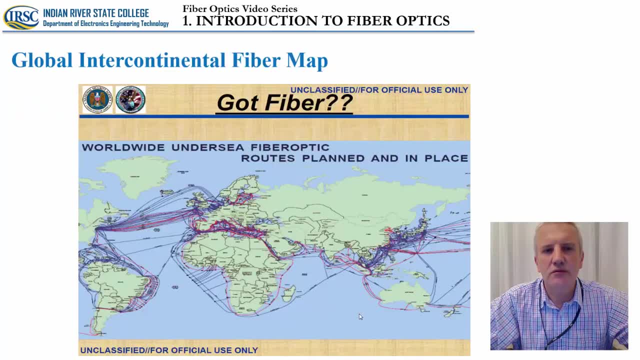 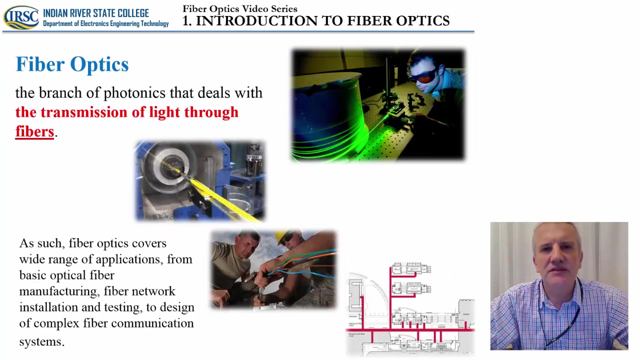 And finally, this slide here gives a brief glimpse of intercontinental fiber optic links that are connecting the continents. These optical fiber cables are being laid on the bottom of the ocean and providing the communication between the different nations on different continents. Now that we briefly introduced the field of fiber optics and all immense opportunities it offers to 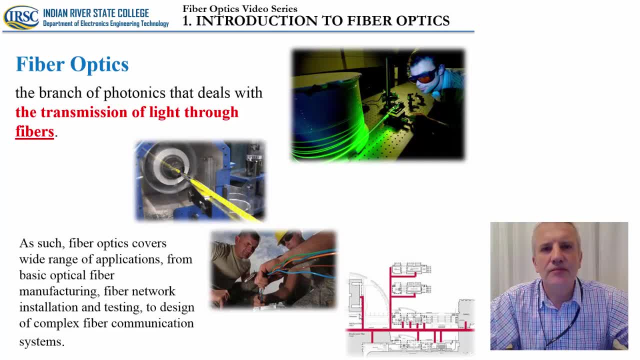 the people who are trained in this field. let's also briefly introduce the field of fiber optics And all immense opportunities it offers to the people who are trained in this field. Let's also briefly tour our fiber optic lab to expose you to the equipment that you're going to be trained on. 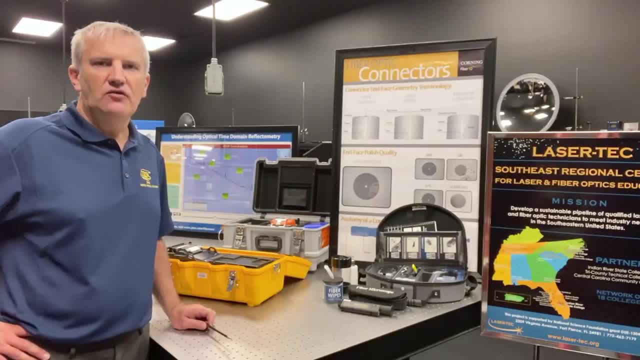 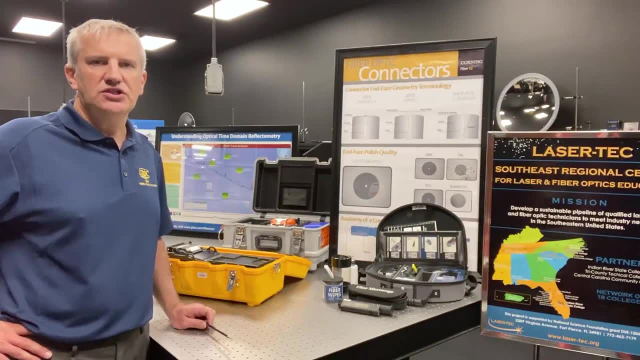 during the practical portion of this course. We are here in our photonics lab at Indian River State College main campus in Fort Peace, Florida. My name is Mohan Sanovic and this is a short video in which I'm going to introduce equipment that we are going to use in a practical portion of this. 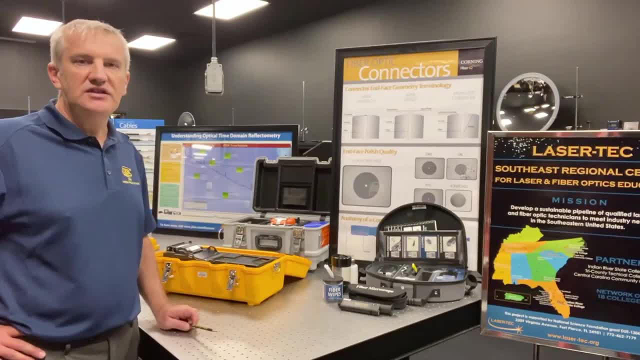 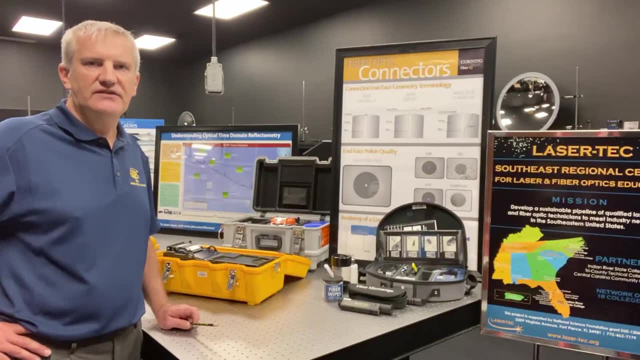 course, All the equipment that we are going to be using is an industrial equipment, meaning you're going to be trained on the equipment that you're going to be using out there in a fiber optic field As a fiber optic technician. we are going to be using the tools and equipment and devices from 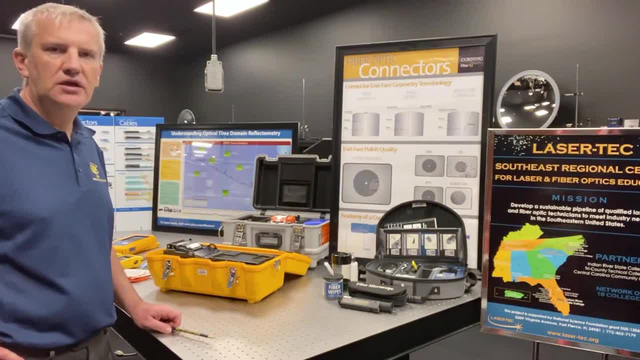 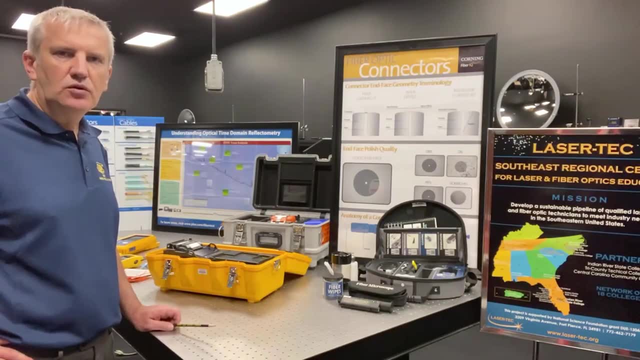 the market leaders in this field, such as Corning, Fluke and similar. And again, what you're going to come across in this practical portion of the course is actually going to be the equipment that you're going to use out there in your career or on your job as a fiber optic technician. 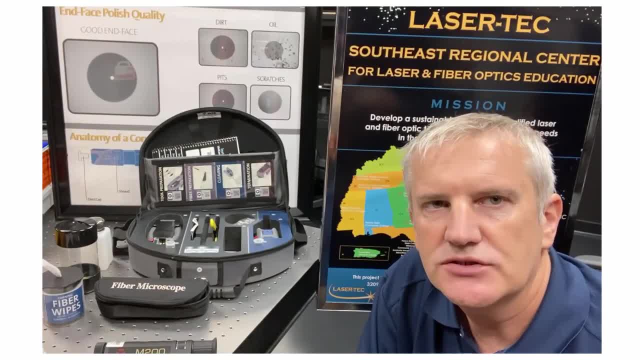 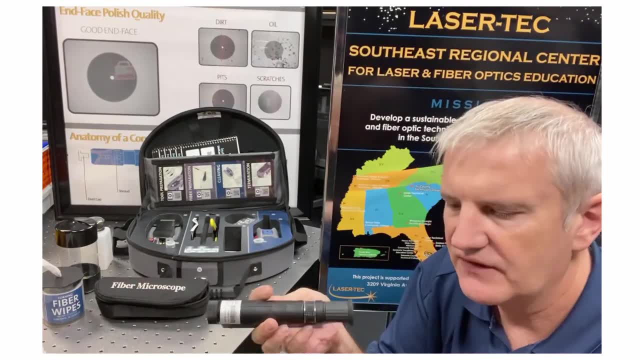 In the first few lab experiments. in the hands-on portion of this course, we are going to be focusing on the optical connectors. First, we are going to be learning about how to inspect the end face of the connector. We are going to emphasize the importance of the cleanliness of 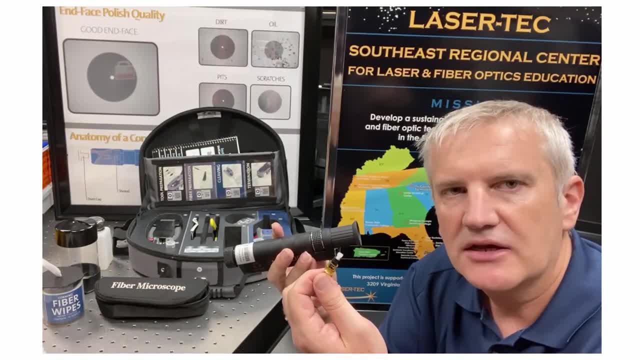 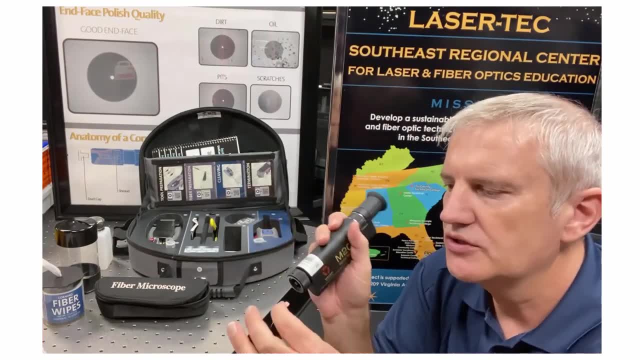 the end face of the connector and negative impact of the dirt on the end face on the optical losses. And then, as a practical portion, you are going to be learning how to visually inspect using some of these tools, such as this small optical microscope made by Yamasaki. 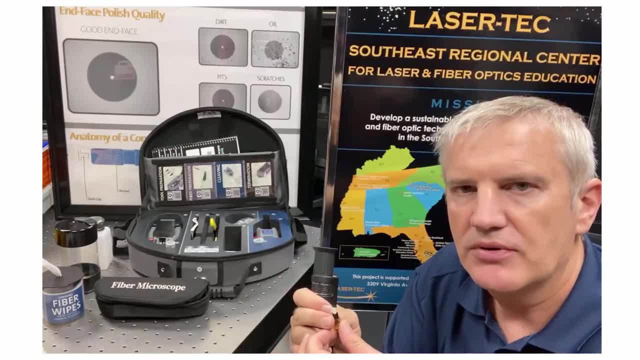 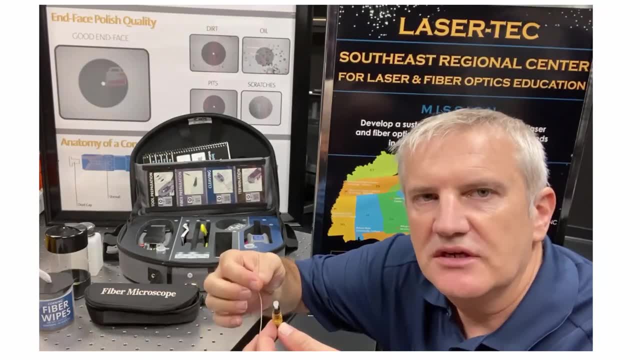 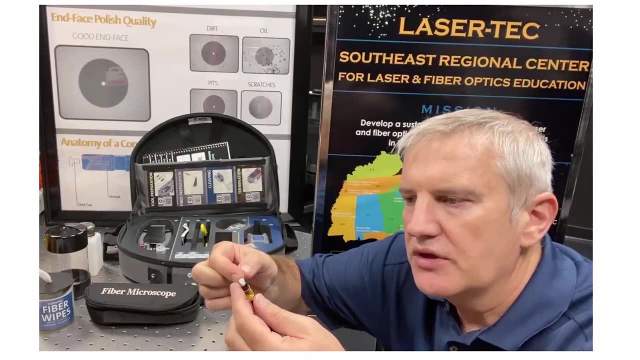 So you're going to be inspecting the end face and then also learning proper procedures for both the dry and wet cleaning of the end face of the connector. One of the important skills that you would want to develop as a fiber optic technician is also properly installing the connector onto the optical fiber. We are going to be talking. 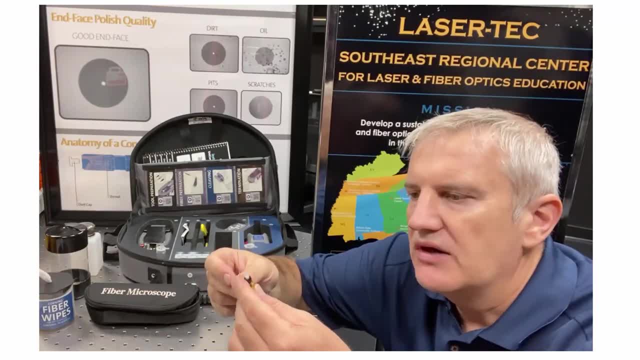 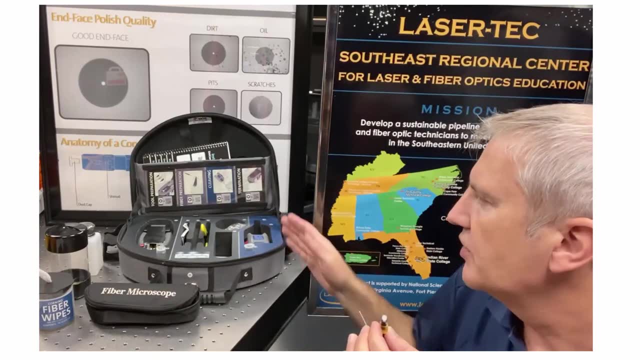 about a few different techniques that are used to mount the connector, such as anaerobic method and a few other, And then we are going to be introducing this UNICAM Corning kit that you're seeing here that we're going to be using in a hands-on portion of the connector in 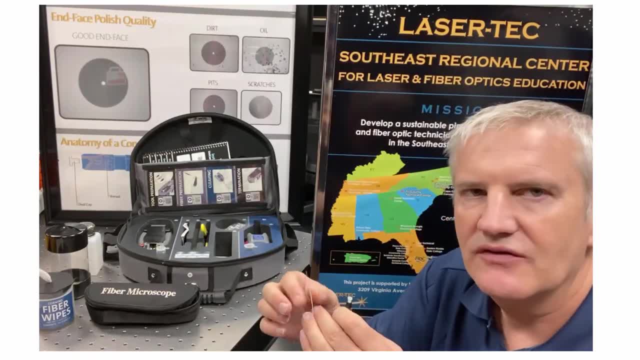 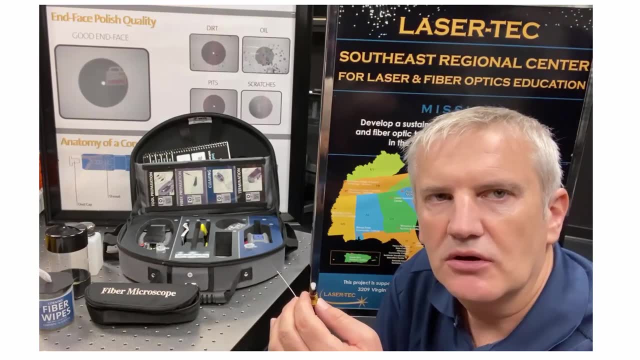 the future And we're going to be using this as a guide to the installation. So you're going to learn how to properly establish the end face of the fiber and properly install it in the connector so that you avoid any kind of air gaps that may result in optical losses. So you'll be introduced. 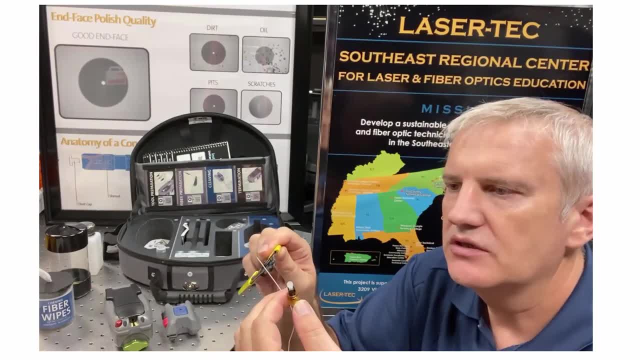 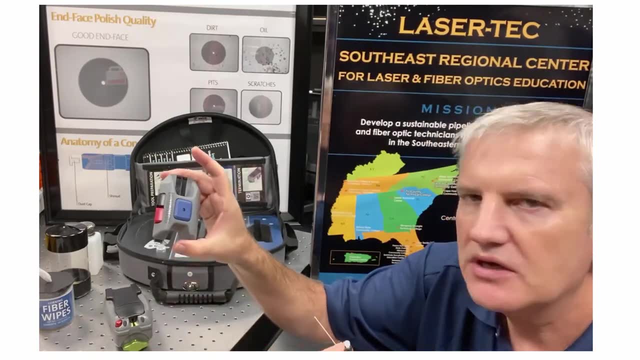 to the tools, such as the wire strippers, to be used to remove different layers, including the buffer, as well as the coating on the optical fiber. You're going to use this small tool here to properly cleave the fiber. And then, finally, the last tool. 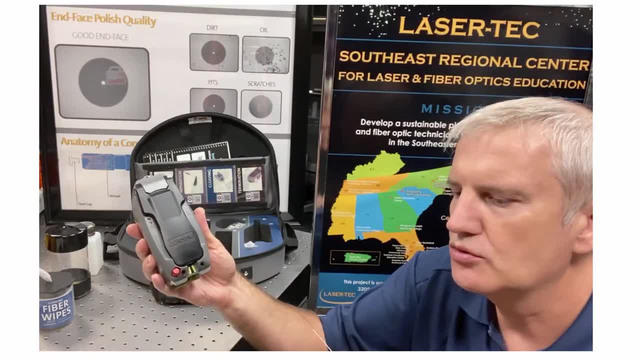 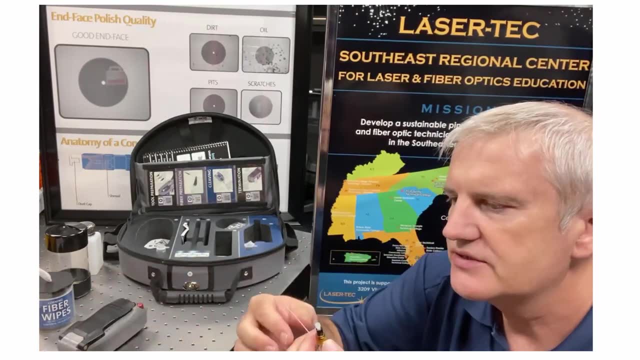 the first part of this UNICAM kit is the tool to be used to properly install the connector onto the optical fiber. So this is going to be a lab that's going to take a few hours, during which you're going to be practicing the way to properly prepare optical fiber, the end face of the optical 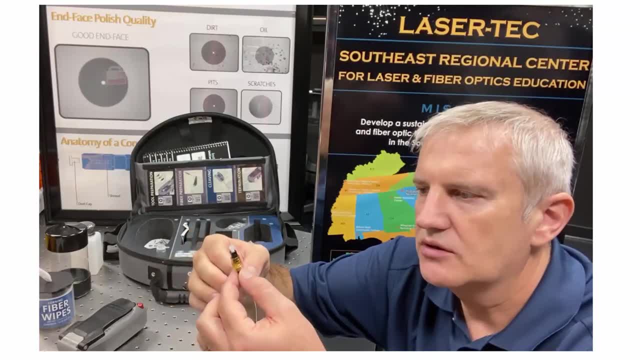 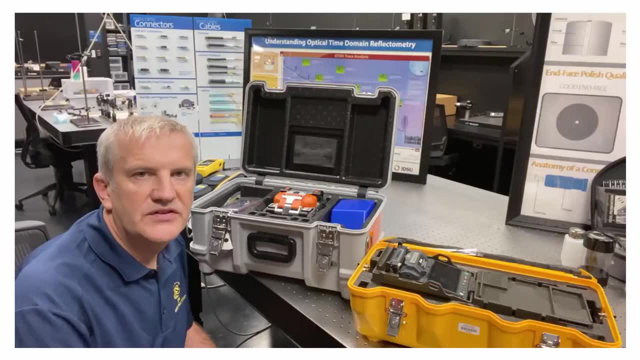 fiber, to properly cleave it and then finally, to install the connector in the proper way that would minimize the loss as the interface between the optical fiber and the connector. And then the next portion of the hands-on experience is going to be fiber optic splicing. So we're going to be learning how to splice two fibers. 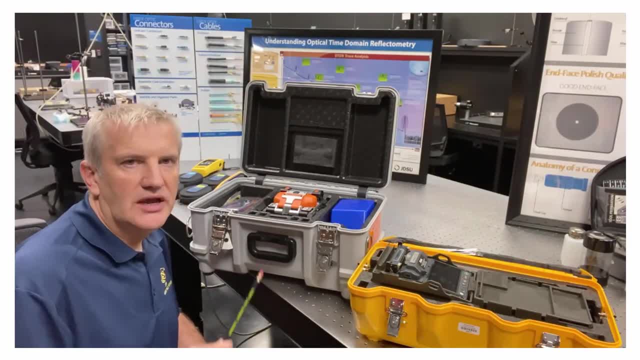 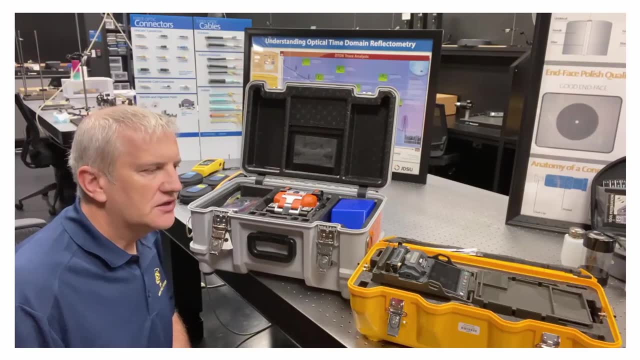 You're going to be using these two splicers here, one made by Fujikura and another one made by Sumitomo, So these are industrial type of fiber optic splicers. So you're going to learn how to properly prepare the end faces of the two fibers and then how to properly mount them into the 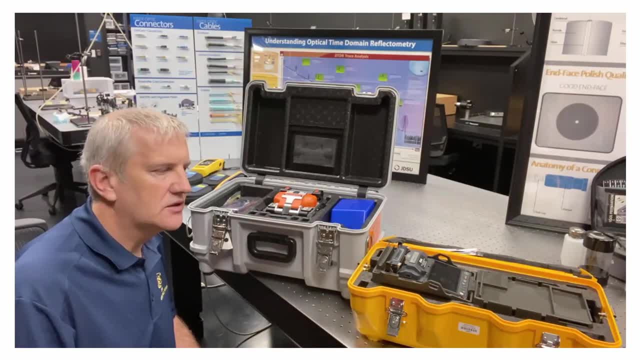 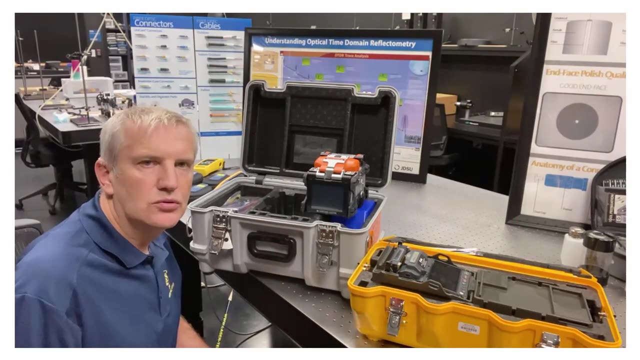 fixture on each of these two fiber optic splices and, finally, to perform the fiber optic splicing as well as the installation of the plastic protective buffer. Both of these fiber optic splicers have a nice small screen that are going to enable you to monitor fiber optic alignment during the process of splicing, as well as the process of splicing. 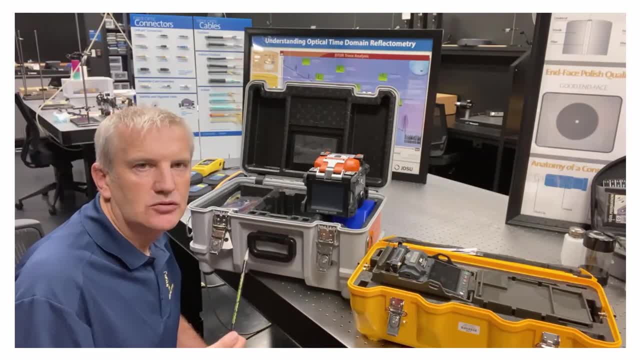 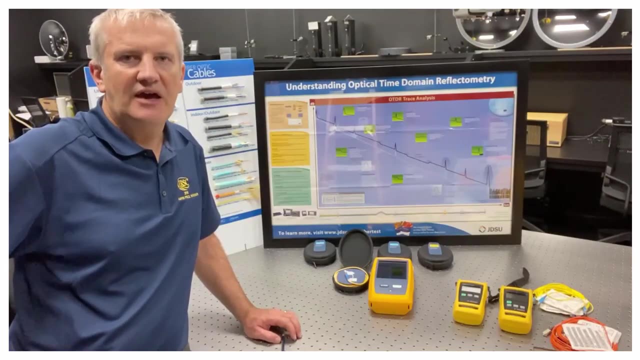 when the arc is being produced and the two optical fibers are spliced. So this is an important skill that you're going to develop on this industrial type of fiber optic splicers, during the practical portion of this course And then, finally, in the second half of the hands-on course, you're going to 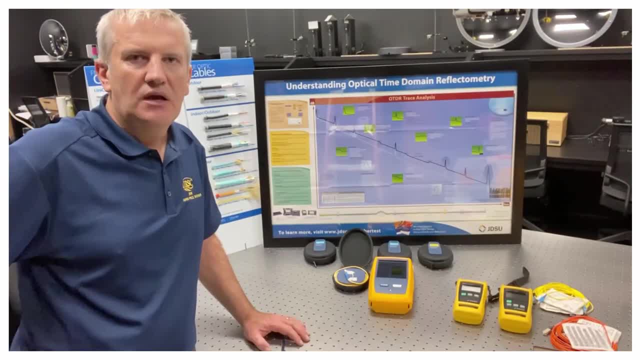 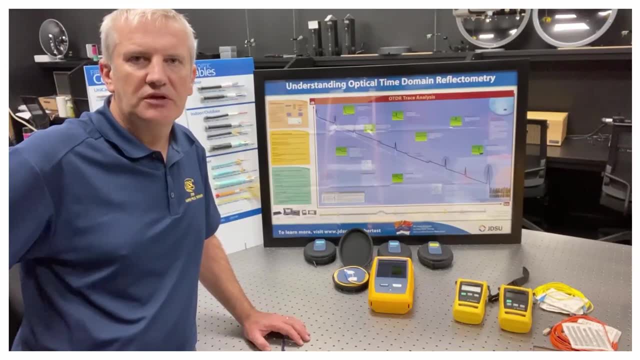 be performing fiber optic measurements. After learning how to install the connector and how to properly splice the two fibers, you're going to be establishing your small fiber optic links with the two connectors on each side and then performing different types of measurements. You're going to 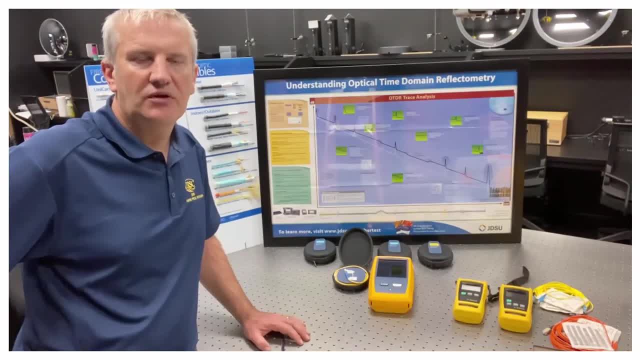 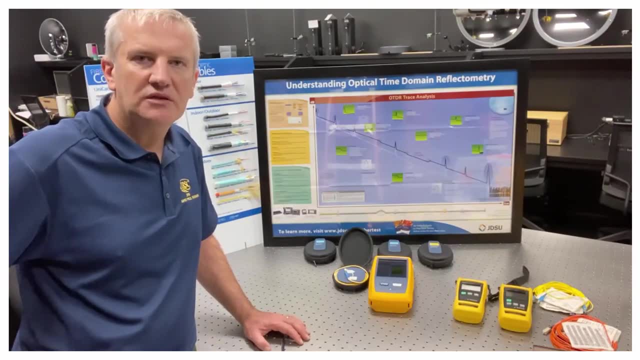 emphasize the importance of accurate and reliable measurement and then move over to the practical portion of the fiber optic measurement. We're going to be performing two measurements, tier one and tier two. The tier one measurement will be conducted using optical source and optical meter by the manufacturer. 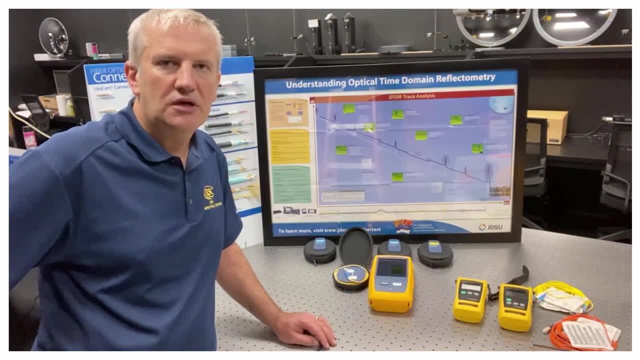 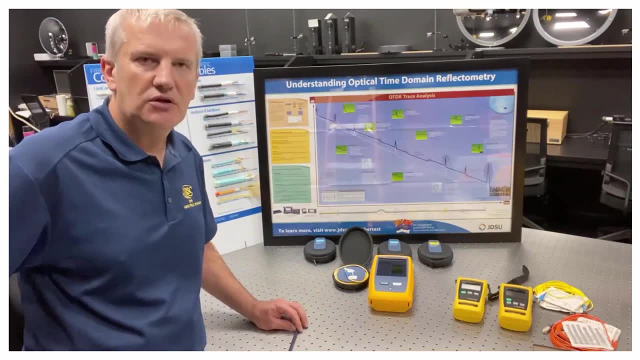 We're going to be characterizing the optical loss over the fiber optic link in terms of the optical loss, and then we're going to move over to the optical time domain, reflectometry, or tier, two measurements that we're going to be performing on a Fluke: optical OTDR or optical. 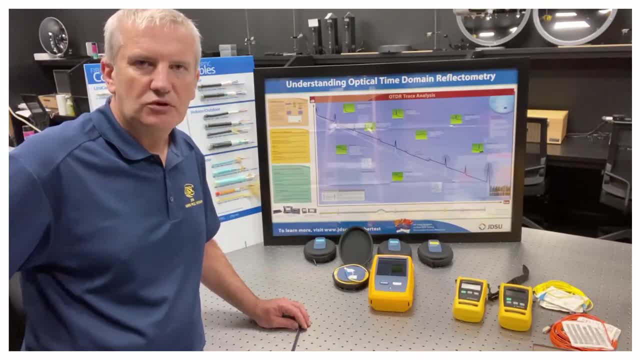 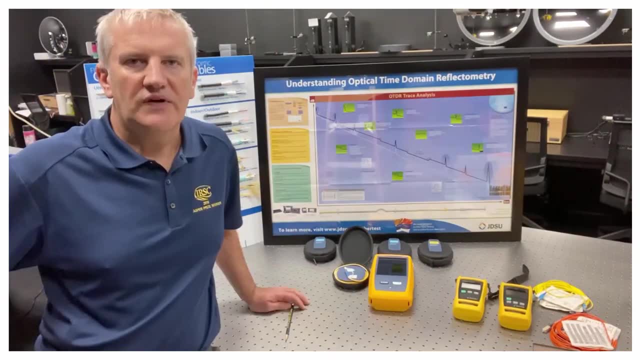 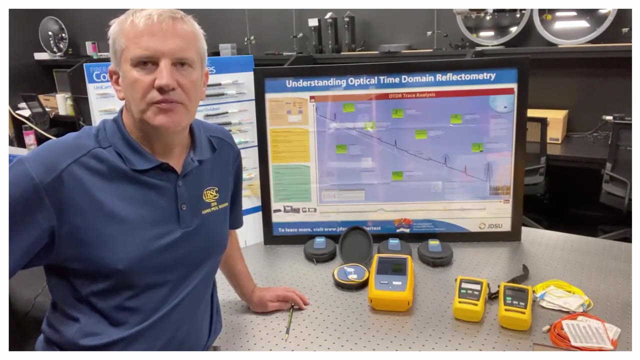 time domain reflectometer. So we're going to be introducing the whole concept of optical time domain reflectometry and its advantages over the regular T1 measurement And, once you're introduced to all these different types of measurement devices, we also have a replica of the real fiber optic link here at the main campus of 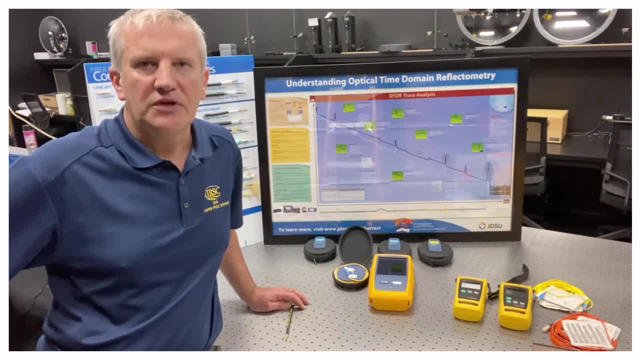 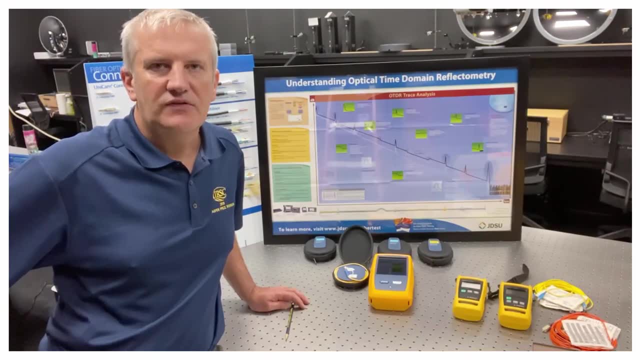 Indian River State College. On that replica of the fiber optic link. you're going to be performing real-time measurements of a few different types of fiber optic clicks and different scenarios. Some of the fiber optic links will be damaged. they will be of a different length. 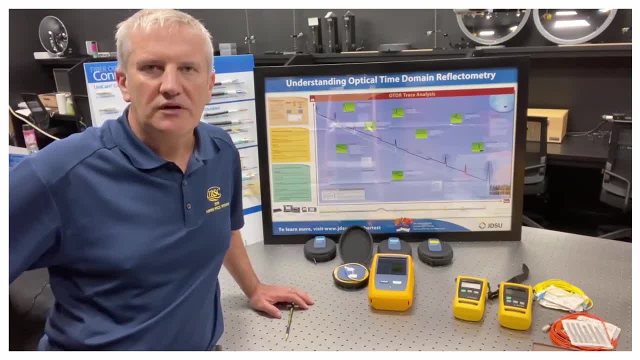 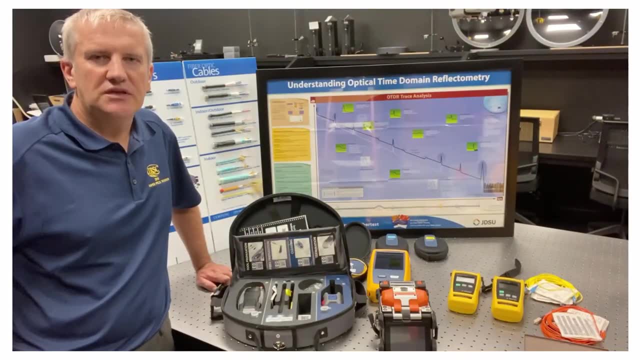 so you would be using some of this equipment to properly characterize fiber optic link of different lengths and different scenarios on it. So this is a short overview of the equipment that we're going to use in a hands-on portion of this course. This is the most fun part of the course. 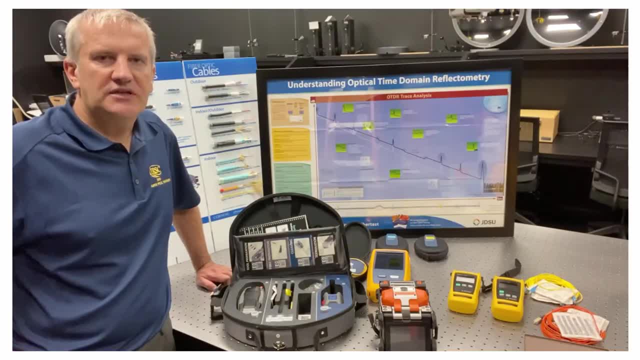 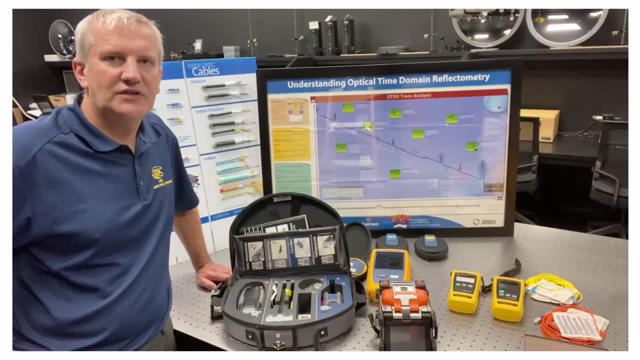 through which you're going to have an opportunity to learn and develop the skills of a fiber optic technician- hands-on skills, and at this point, I'm looking to seeing you all here at the main campus of Indian River State College. Now that we briefly introduced the fiber 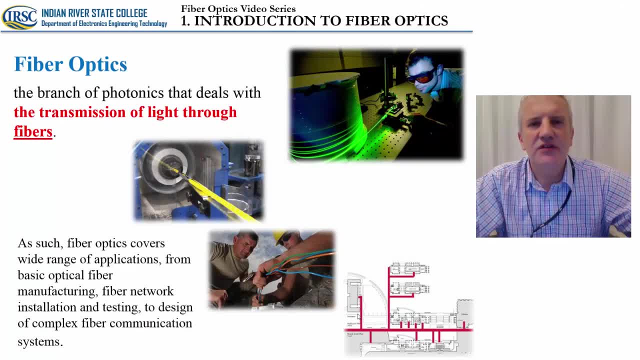 optics course, as well as a hands-on portion of it. let's start with the theory. In this first lecture, we are going to review some of the concepts that have been covered in the previous course, so let's see what are the basic properties of light and how they can be applied to the 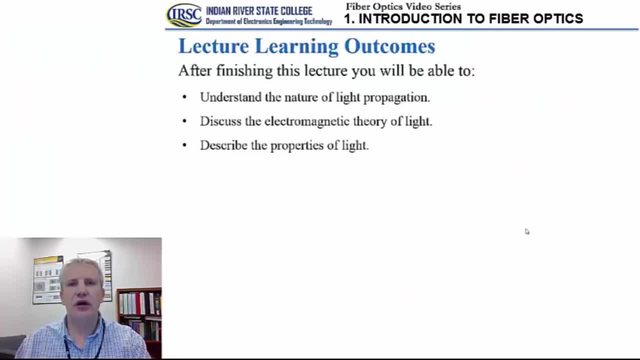 field of fiber optics. There are a few learning outcomes that we need to achieve today. As a result of this lecture, you should be able to understand the nature of light propagation, at least on the basic level. We're going to spend some time discussing the electromagnetic theory. 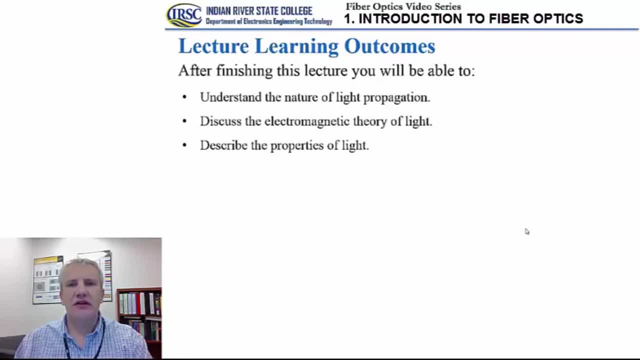 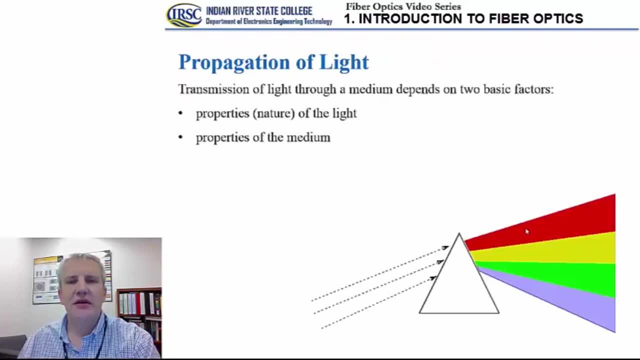 of light and, finally, we're going to spend a significant amount of time talking about different properties of light. In the field of fiber optics, we are using light as a medium that carries information along some sort of guiding structure, which, in this case, is known as optical fiber. So, in order to properly understand the behavior of light along optical 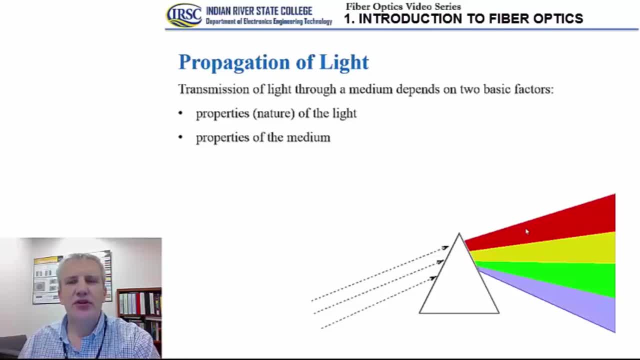 fiber. we are going to start this review of the basic properties of light by discussing the propagation of light and some of the important factors that would determine the behavior of light in a specific medium. So there are two basic factors that need to be analyzed and understood. 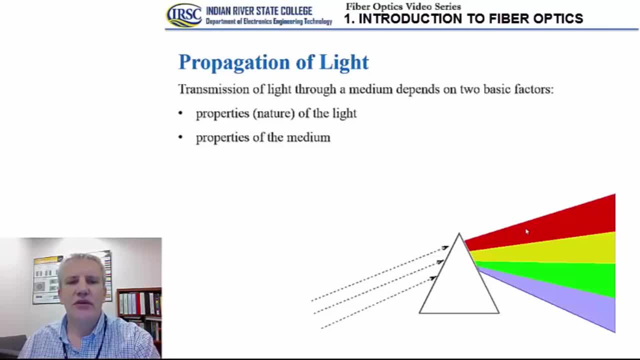 One are the properties of the light and another one are the properties of the medium. So the medium is a supporting structure and light is going to be a carrier of the information that is going to travel through that medium. So there is going to be certain interaction between the 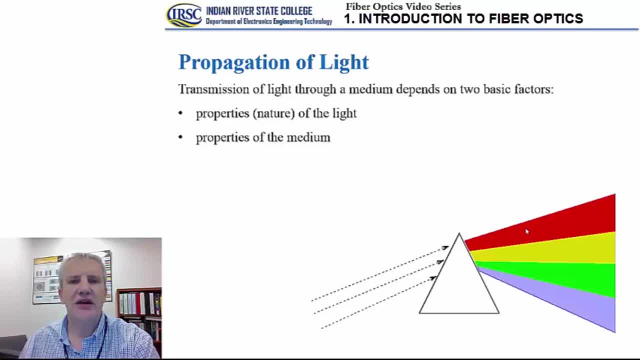 light as an information carrier on one side and the medium as a supporting structure to which light is going to propagate. So we are going to visit each of these two basic aspects of the light propagation and try to understand how they affect the behavior of light and its information capacity. 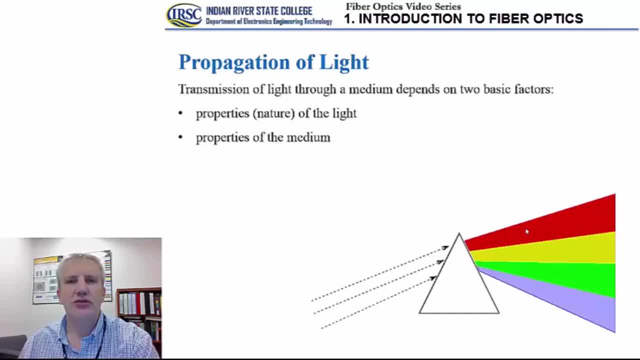 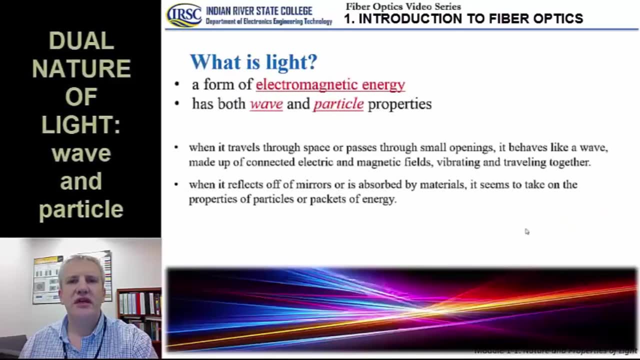 when light carries information, either in a free space or, specifically in the case of fiber optics, as the light propagates along an optical fiber. In order to understand the basic properties of light, we are going to start with the basic question of what is light? This question, 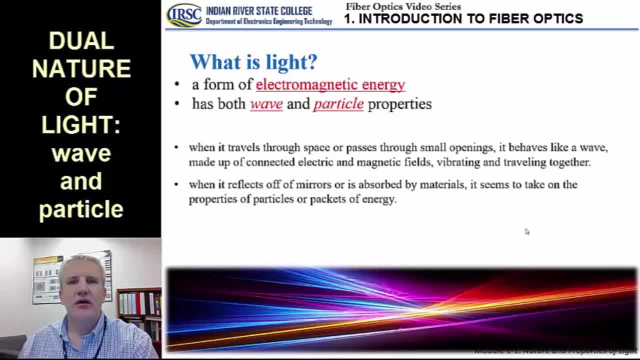 preoccupied many scientists throughout the history of science, and today, at this level of knowledge, we are looking at the light as a form of electromagnetic energy that has both wave and particle properties. It turns out that certain phenomena that are related to the light can be explained only if you're looking at light as a wave. 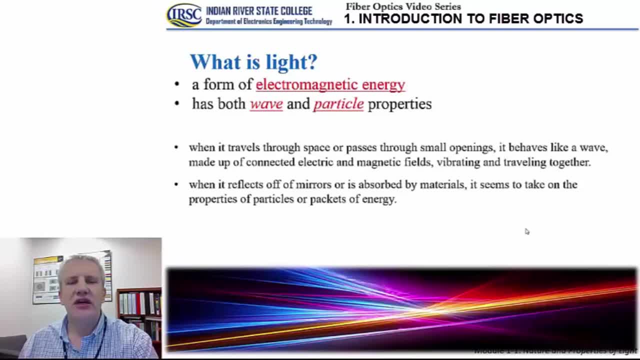 while some other phenomena can be explained only if we are looking at the light as a form of electromagnetic energy, or light as consisting of many small particles. So, for example, when the light travels to the space or passes through small openings, it is going to behave like a wave similar to like water waves or sound waves to a certain level. So, in other words, 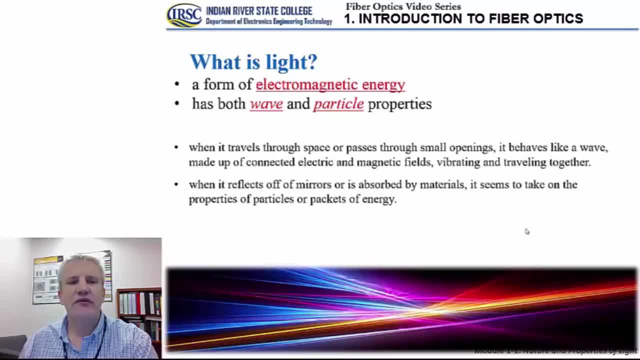 light is gonna behave like as if it's made up of connected electric and magnetic fields that are vibrating and traveling together. On the other side, there are other phenomena that cannot be explained. explain by looking at light as a wave: Certain phenomena such as absorption, in other words, 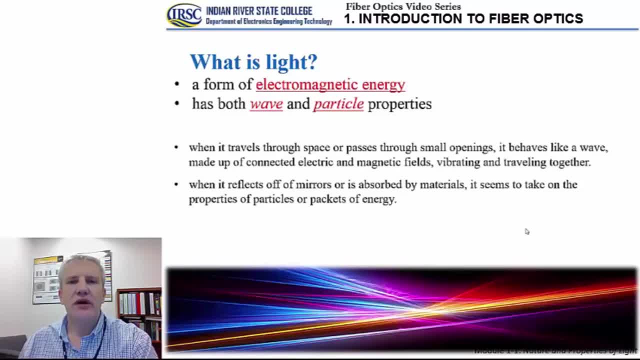 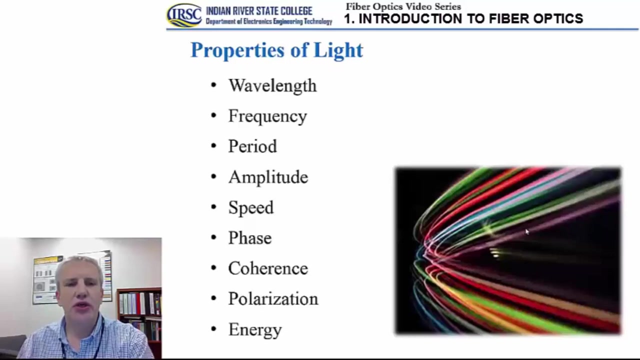 the way how the light is interacting with the medium by reducing its power and transferring its energy onto the medium, can only be explained if you're looking at the light as a whole bunch of small particles that are interacting with the particles of the supporting medium. This slide here lists important parameters that are going to be used to describe the 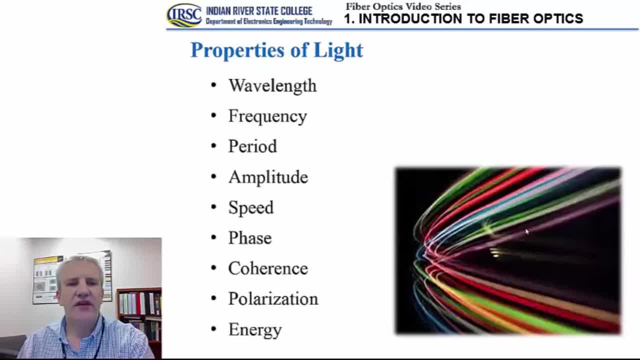 properties of light. The most important are the wavelength, the frequency, the period, the amplitude, the speed of light, the phase, and also the coherence, the polarization and, finally, the energy of light. On the slides that follow, we are going to discuss each. 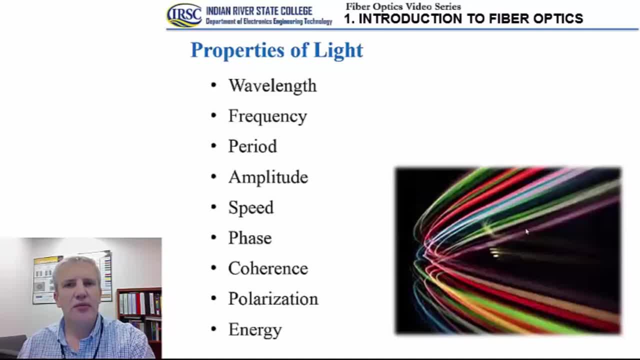 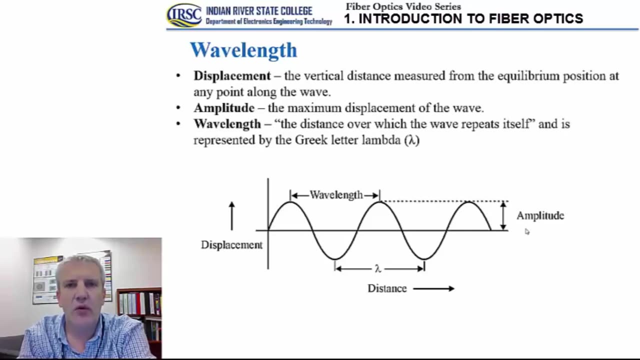 of these parameters individually and we are going to try to properly understand them, as they play a very important role in the field of photonics. Let us first talk a little bit about the wavelength. We have already mentioned that light behaves as an electromagnetic wave. What do we mean by wave? What is a wave? How can we define? 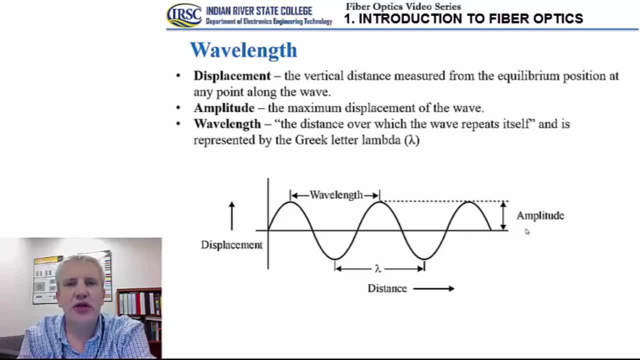 a wave. A simple explanation is that you can look at a wave as some sort of disturbance that takes place, that occurs both in the space and in time. For example, if you're looking at the water waves. if you look at the waves, 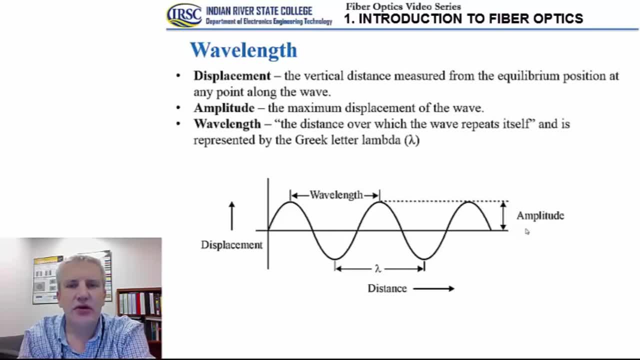 the ocean, you are going to look at the disturbance. you're going to look at the peaks and valleys that are distributed along the space. In other words, at different locations you're going to have a peak or a crest, and at some other locations you are going to have a valley. 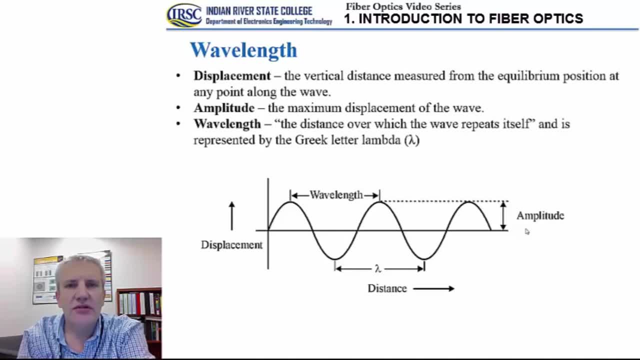 or the minimum. Similar disturbance, similar vibration, also occurs in time. For example, if you are anchored in a boat at the same location, over time that boat's going to be moving up and down. So at certain points in time you're going to be at the peak or at the crest, and then at some other time you're going. 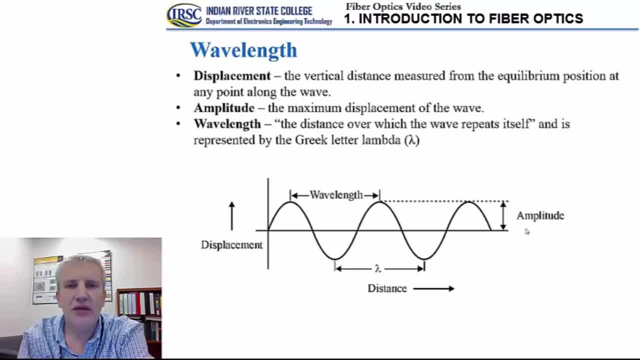 to be moving down into the valley or at the minimum position. So that's what we consider a wave. In order for a wave to be a wave, there has to be a disturbance, both in space and in time, And that disturbance can be a disturbance of different. 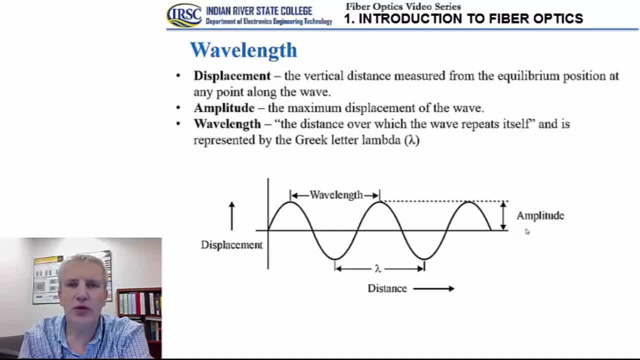 types of quantities. If we are looking at an ocean wave, we are talking about disturbance of water. If we are looking at a sound wave, then we are talking about disturbance of air molecules. In this specific case of light, we are talking about an electromagnetic wave. We're talking about 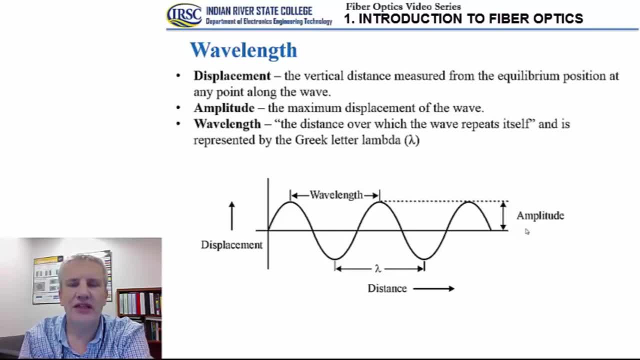 a disturbance of so-called electric field and magnetic field. You can, to a certain extent, correlate electric field to the voltage and magnetic field to the current. So if you're looking at a light as an electromagnetic wave, we are talking about a disturbance of the current and the voltage in space and in time. 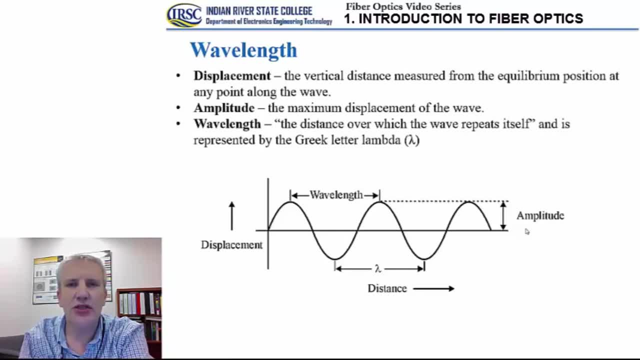 So in order to properly describe that disturbance, that change from a minimum to a maximum in space and in time, we are going to use different parameters to describe those. One of the parameters is a wavelength. So what you see here on this slide on the bottom is some sort of wavy or 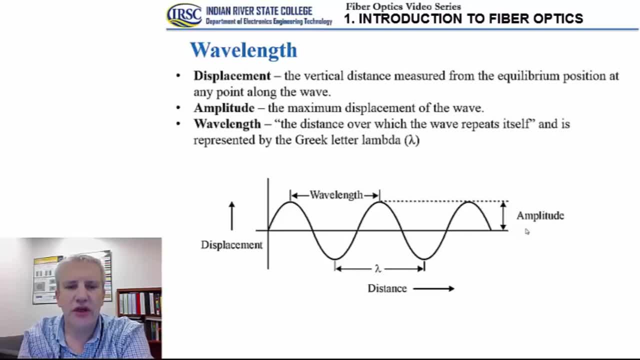 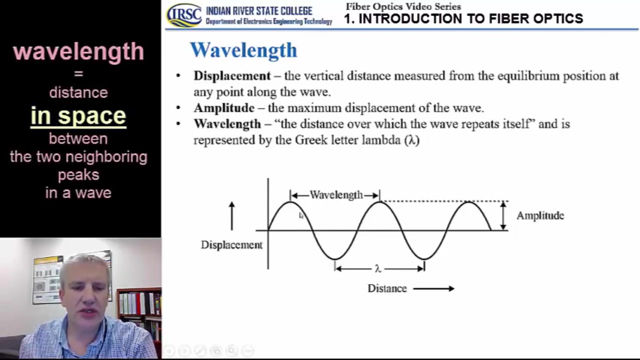 if you want to be more specific, sinusoidal curve, where you can notice a whole bunch of peaks, positive peaks or crests, and also a series of negative peaks. The wavelength is defined as the distance in space between the two neighboring crests, between the two neighboring peaks. So if you're 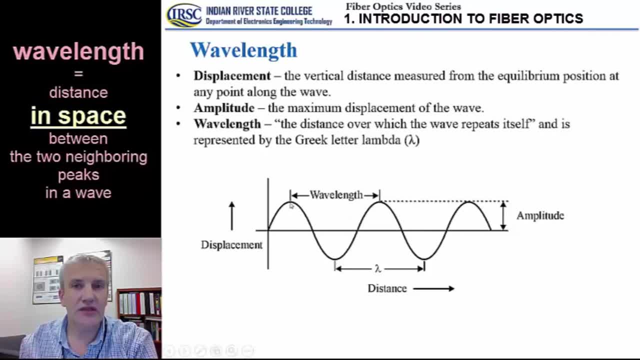 measuring the distance in space. we said that a wave is a disturbance in space in addition to being a disturbance in time. So in this case, here we are considering disturbance over the space. That's why, along the x axis, we are using a parameter of distance. So if you're measuring the distance in space between 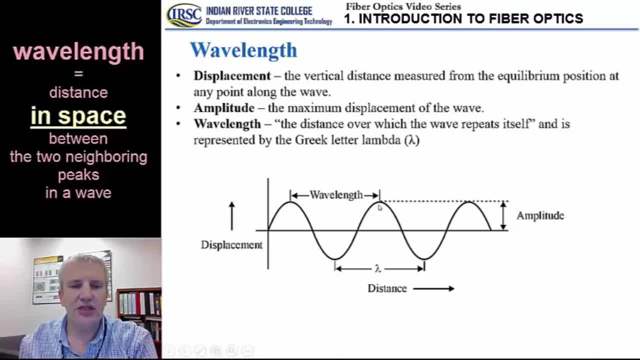 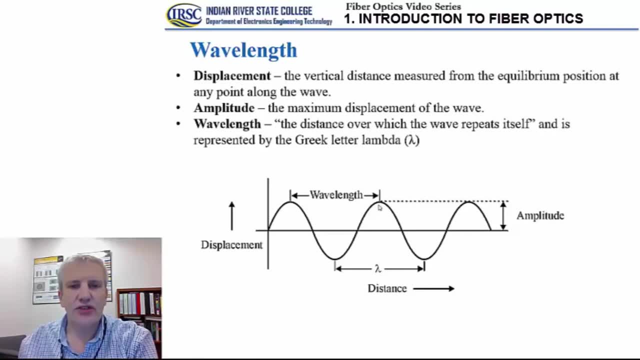 the two crests or the two peaks. that distance is so-called a wavelength. That's how we are defining the wavelength. So the wavelength represents again the distance over which the wave repeats itself. Distance in space. We are using the Greek letter lambda to describe the wavelength and obviously the units that. 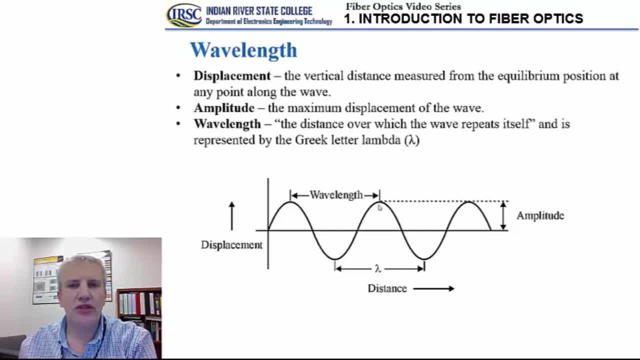 are going to be used to describe the wavelength are going to be units of distance, be it meters or smaller units such as micrometers in the case of light, nanometers. Of course, you can also use British units, you can use inches or mils, etc. So, again, the wavelength represents the parameter that describes. 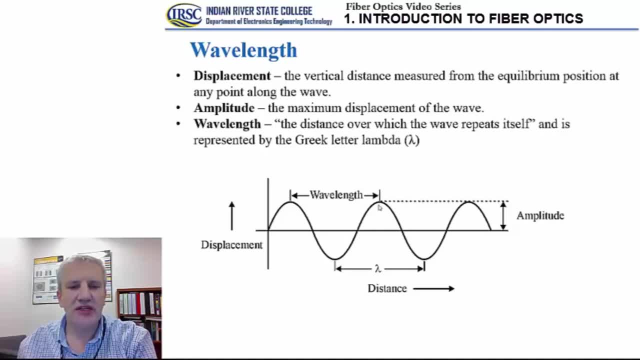 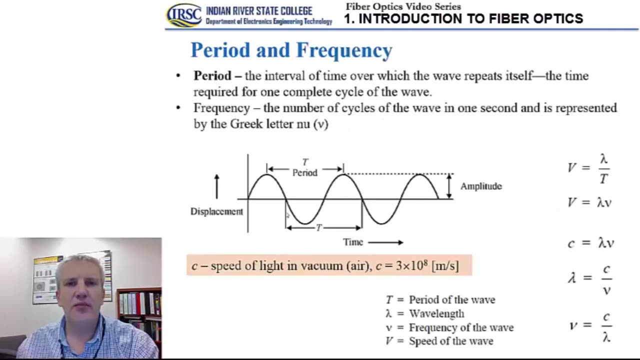 the distance in space between the two crests or two peaks or two maxima in some sort of wave, in this case light, as an electromagnetic wave. We have already elaborated the wave behavior of light and we also define the wave as a magnetic wave. 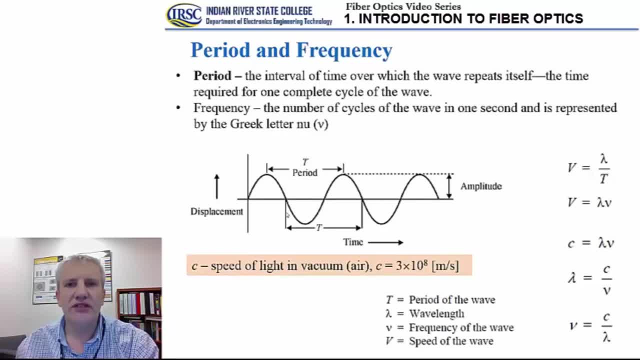 We define the wavelength as a disturbance of a certain quantity, both in space and in time. On the previous slide, we were focusing on the disturbance in space and we defined the wavelength as the distance in space between the two peaks or the two maxima of a wave. On this specific slide, we are shifting the gears to time. 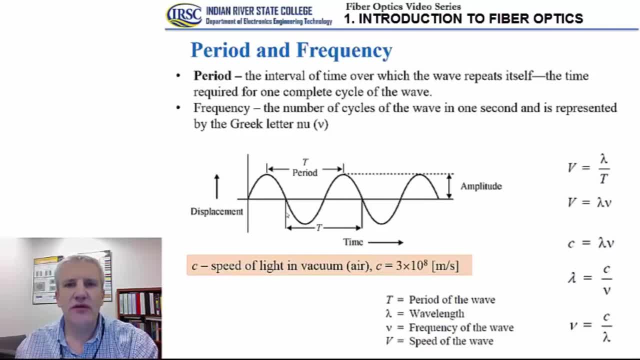 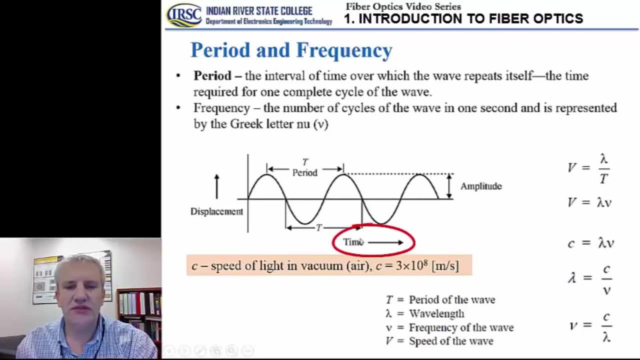 domain. in other words, we are talking about the disturbance or vibration in time. So we are still dealing with the, with a similar wavy or sinusoidal curve, but the fundamental difference here is that along the x-axis we are representing the time, as opposed to the. 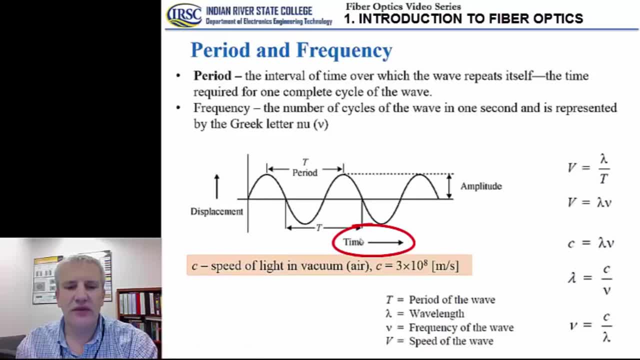 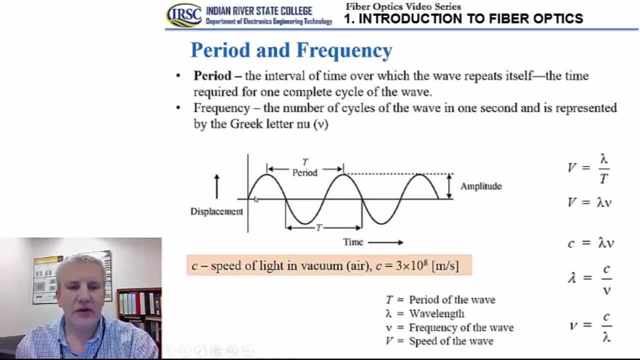 space or the distance that we had on the previous slide. So what we can observe here is that over time the value of a certain quantity, in this case electromagnetic field, is going to be changing from the positive peak to the negative peak, to the positive peak to the negative peak, etc. So we are having a 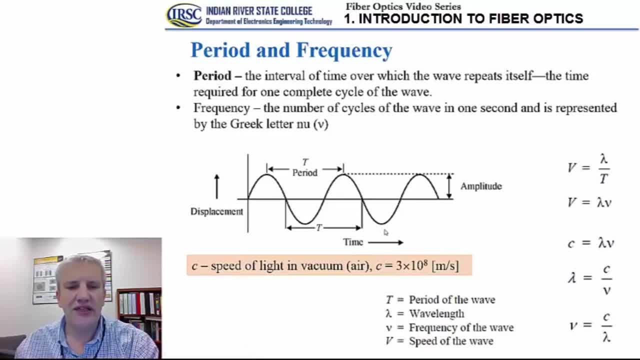 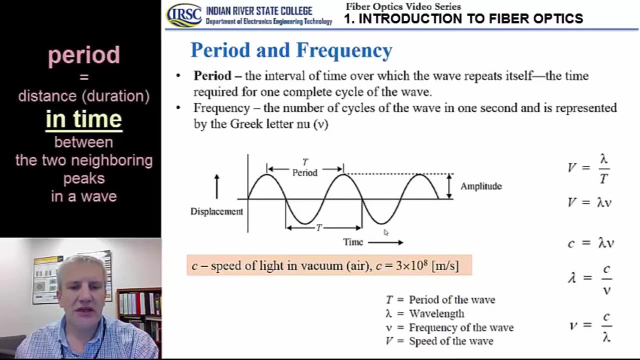 disturbance or vibration of electromagnetic field over time, and the parameter that is going to describe this behavior in time, this oscillation in time, is going to be the period. So the period is basically the distance in time between the two peaks. In other words, if we are measuring how much it takes to 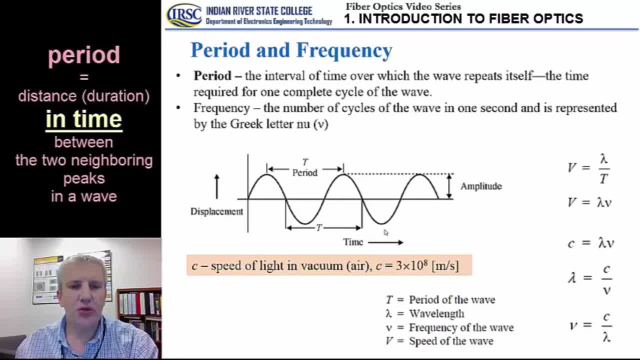 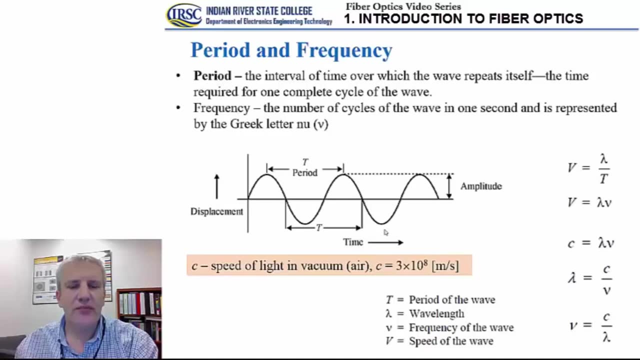 go from one positive peak to the next positive peak. that duration is going to be defined as a period. The number of cycles or number of the peaks that occur within one second is so-called frequency. So there is a certain correlation between the period and the frequency. The period represents the interval of time over which the wave. 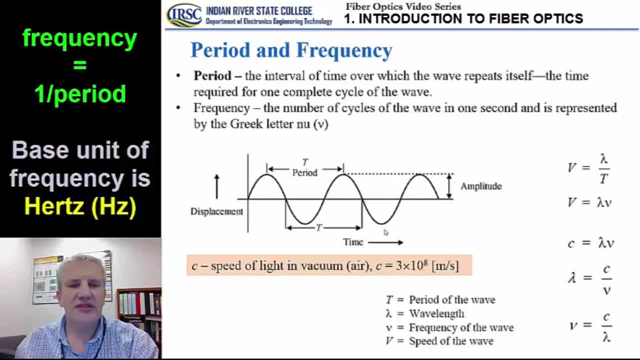 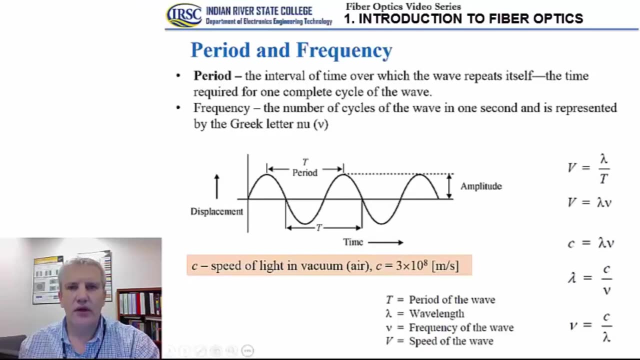 repeats itself. while the frequency represents the number of cycles of the wave in one second, We are using the Greek letter nu, or very often a letter F, to represent the quantity of frequency. At this point, we are also going to introduce another very important parameter that describes the 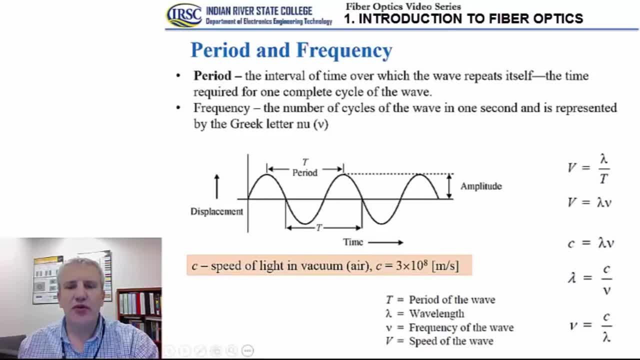 light and that is the speed of light. So light propagates through a specific medium at a certain speed. It turns out that the speed of light is a constant in a specific medium. so if you're looking at a vacuum or air, then the speed of 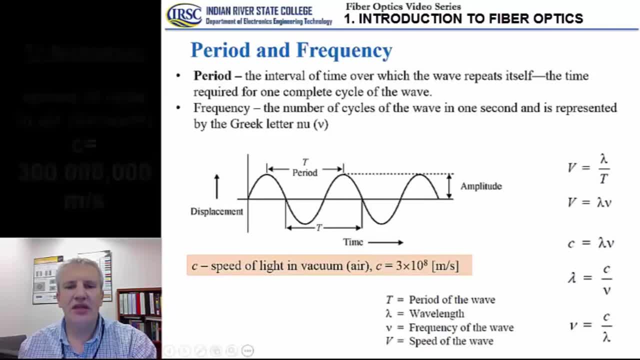 light is going to be equal to 3 x 10, to the 8 meters per second. So that is a constant that is going to be very frequently used in photonics and it's to be remembered. So again, the speed of light, the vacuum, is a constant that is equal to: 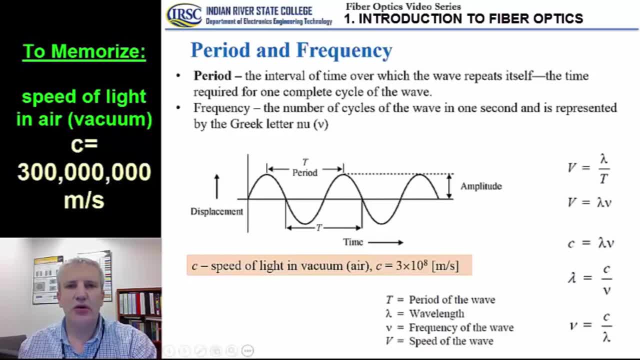 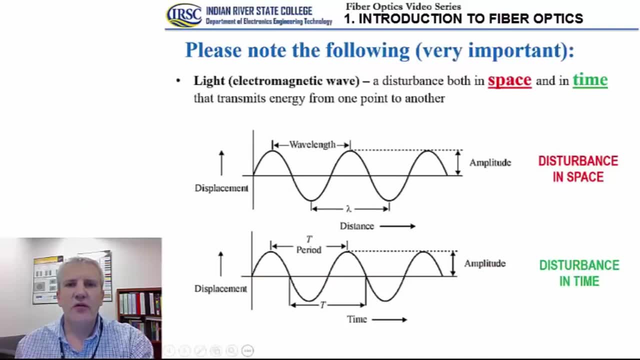 D есть表 to three times 10, to the 8 meters per second or 300 million meters per second. Let us summarize what we covered so far. We have defined a wave as a certain disturbance that takes place both in time and in space. In order to properly 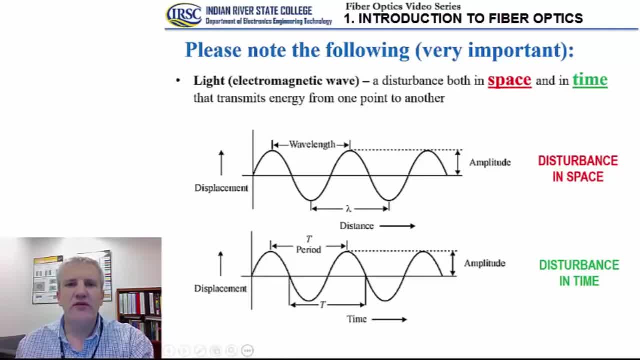 describe the properties of a wave, we are introducing two parameters. We have introduced a wavelength that would properly describe the disturbance in space. In other words, the wavelength is going to be the distance between the two peaks in a wave. And in order to properly describe disturbance in time, we have 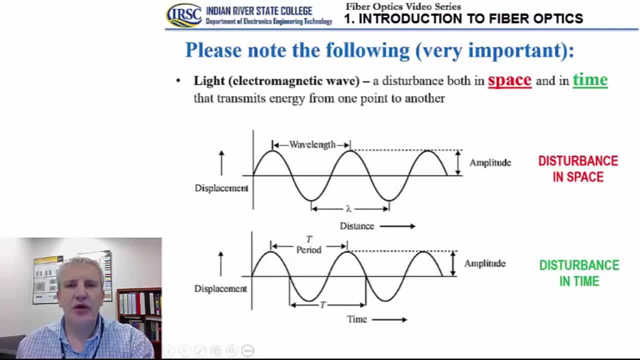 introduced the period as an interval in time to complete one full cycle. We have also mentioned that the light represents an electromagnetic wave. In other words, in the case of light, electric field and magnetic field are vibrating or oscillating in space and time. 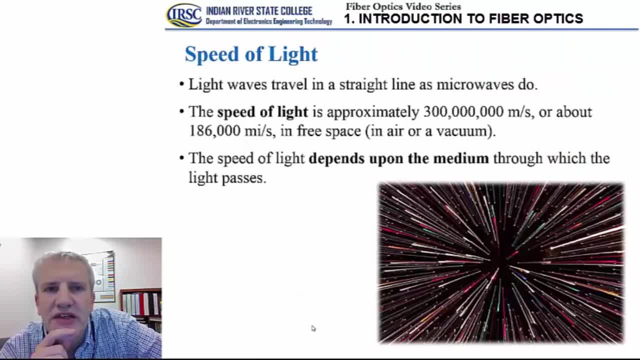 Let us now focus on another important parameter of light, and that's the speed of light. On the previous slides, we talked about the speed of light being a constant and being equal to 300 million meters per second in air or vacuum. It's also 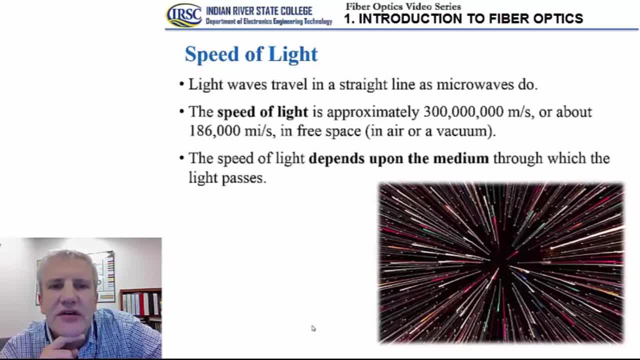 important to mention here that the light travels in straight lines, similar to any kind of other electromagnetic signal, So light pretty much behaves in a similar way as an electromagnetic signal. It's not really a signal that is being used to transfer information from your cell phone. 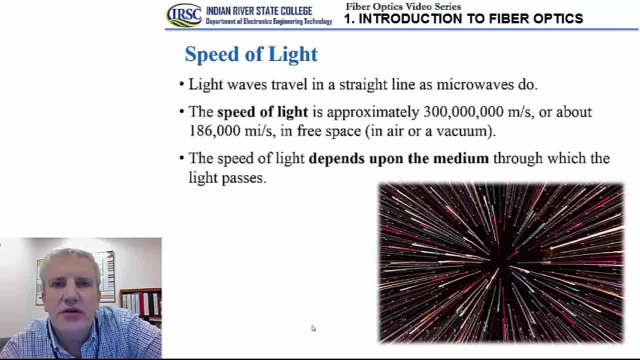 or smartphone to the tower. It's just that the frequency or the wavelength of those two types of electromagnetic waves is going to be the different. So again, the speed of light is approximately equal to three times 10, to the 8 meters per second, or 300 million meters. 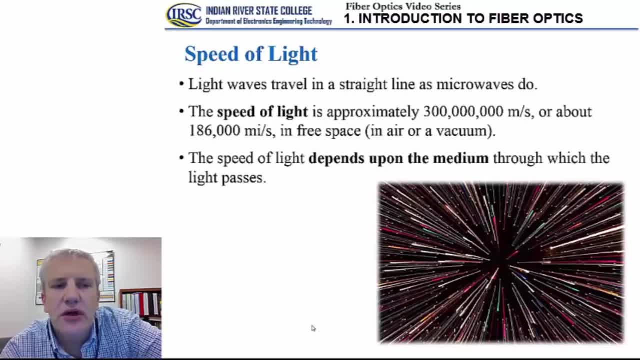 per second Or, if you wish, it is actually equal to 186.8 meters per second. So, if you wish, it is actually 86,000 miles per second. It's important to mention that this is only in the free space, either in the air or vacuum, and that the speed of light is going to. 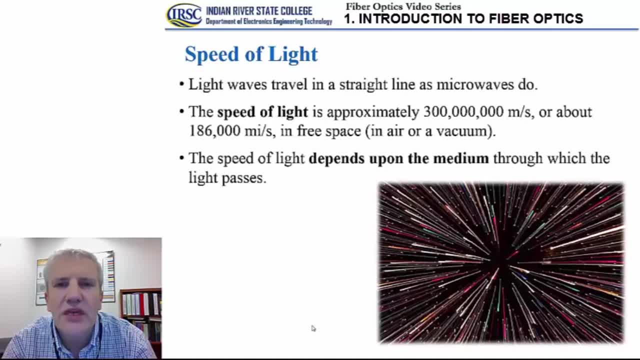 change if the light moves from one medium into another. So the speed of light depends upon the medium through which the light passes. The highest speed is the speed of light in air or in the vacuum, and we are going to see on slides that follow that the light is going to actually reduce its speed if it passes. 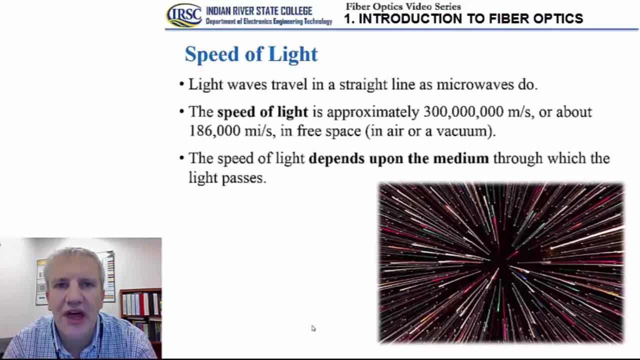 from air or vacuum into some other medium, such as water or glass, etc. So this is very important to understand because it's going to have certain profound effects in fiber optics, since we are using glass as a material to make the core of an optical fiber that is going to be used as a light guiding. 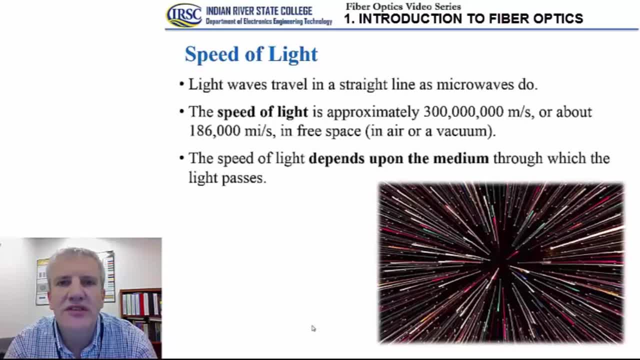 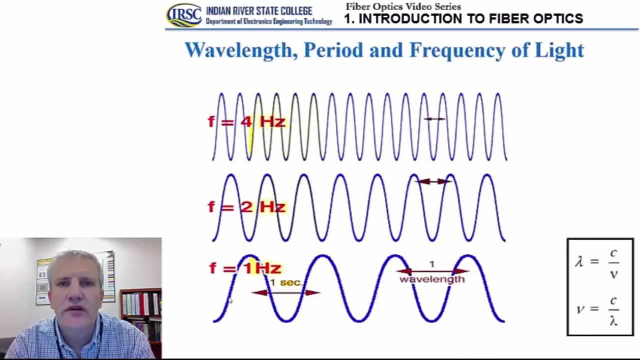 region through which the light is going to propagate and carry information from one side to the other. Here we have a very clear comparison between three waves at three different frequencies. We are seeing a wave at frequency of 4 Hertz on the top and then 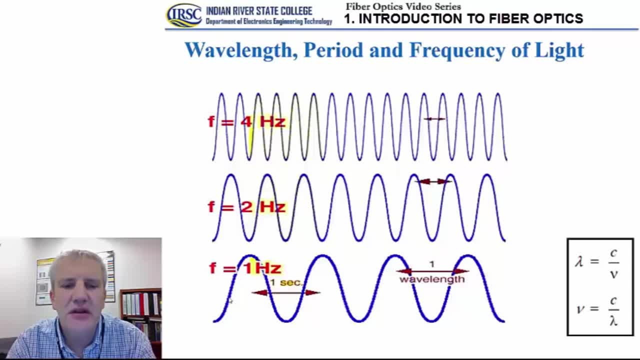 we have a wave whose frequency is 2 Hertz in the middle and finally the wave whose frequency is 1 Hertz on the bottom. So again, the frequency is basically equal to the number of cycles that are going to be transmitted from one side to the other. 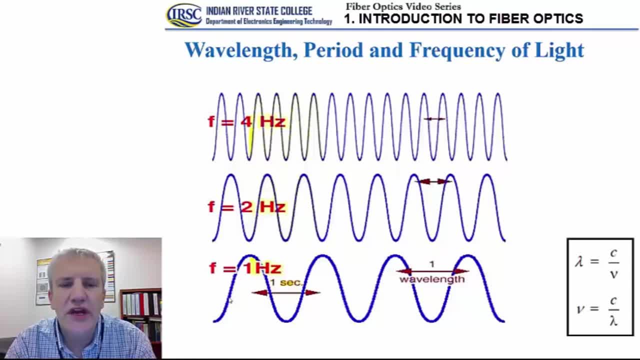 So this is yes. 2 Hertz, as it is shown on the screen and finally as it oneself, is basically equal to the number of cycles completed within 1 second. So 4 Hertz means that four cycles are completed in less than 2 seconds. 2 Hertz means that two. 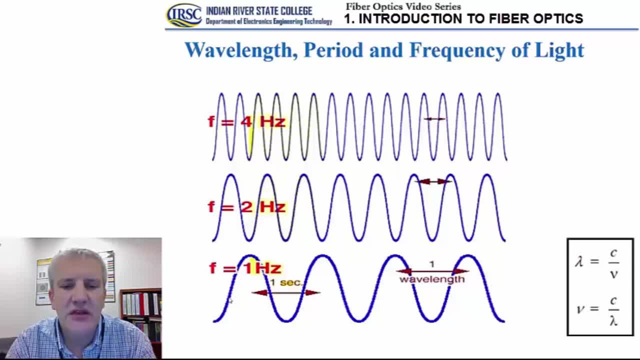 cycles are completed within less than 2 seconds. And finally, the meaning of 1 Hertz is that one cycle is completed within less than 1 second, like we see in this slide, Just like in our video today, that are to be remembered, that very clearly establish the correlation. 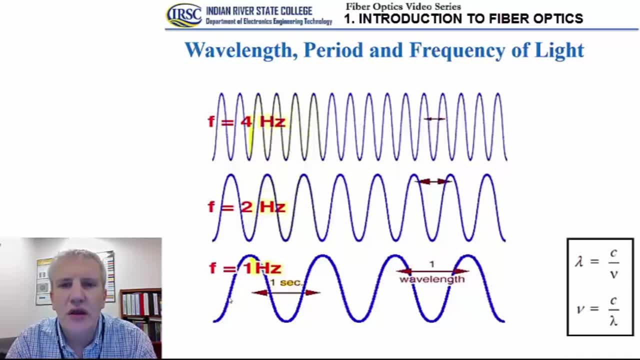 between the three parameters that we have introduced so far: wavelength, the frequency and the speed of light. it's important to mention that these formulas- at this point- you know the way how they have been written- can be applied only for air or vacuum. so, wavelength, we are using the letter of letter lambda, the. 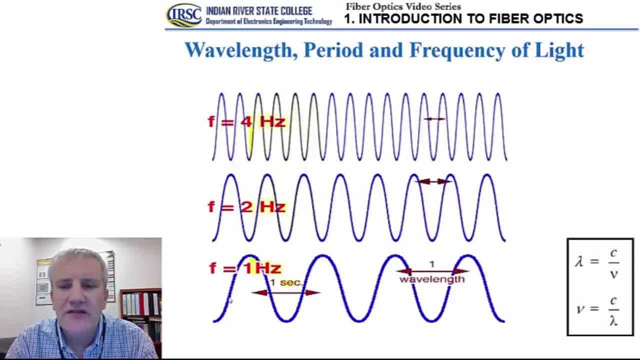 speed of light, you using a small letter C, and finally the frequency- we're using the Greek weather. no, so there is a correlation between these three in the sense that, for example, the first formula on the top basically is stating that the wavelength of light in a vacuum or air is equal to the ratio of the speed of 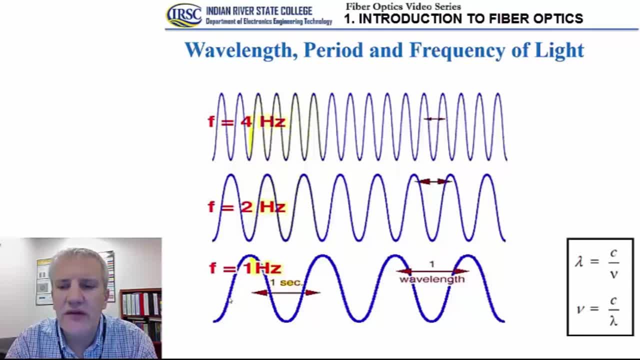 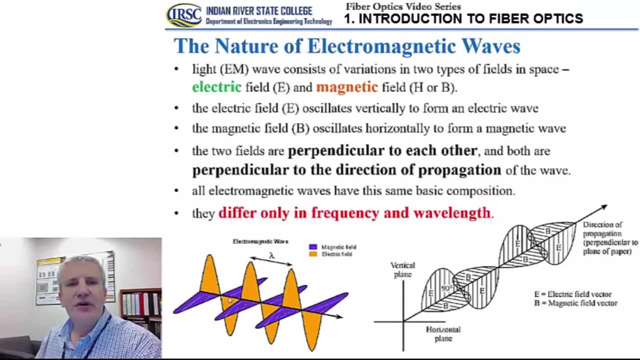 light C and the frequency of that wave of that light: the, the, the, the, the, the. This light dives a little deeper into the whole aspect of an electromagnetic wave. We have already described light as an electromagnetic wave and we said that an electromagnetic wave is a wave where disturbance occurs in space and time and the quantity that vibrates or 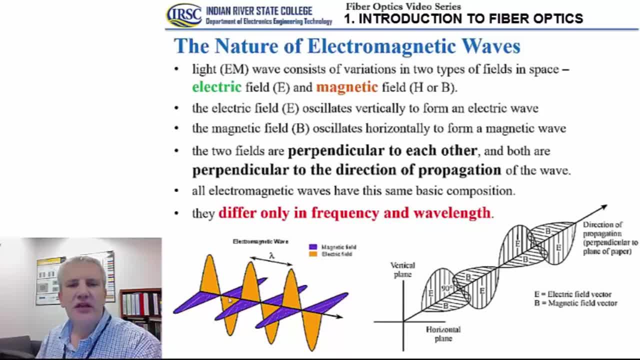 disturbs is electric field and magnetic field. Again, electric field can be looked at as voltage and magnetic field can be looked at as a current. On the bottom of this slide we have a three-dimensional representation of an electromagnetic wave. We said that an electromagnetic wave consists of an electric field and a magnetic field. 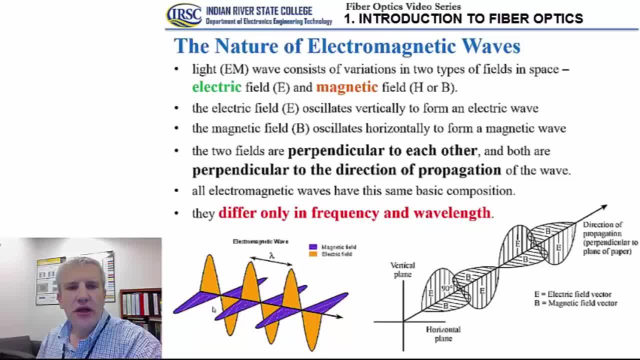 Electric field here is shown in an orange color and it's shown here as oscillating vertically to form so-called electric wave. And then magnetic field is shown here in a purple color and shown here as oscillating horizontally to form a magnetic wave. So these two quantities, electric field and magnetic field, are perpendicular to each. 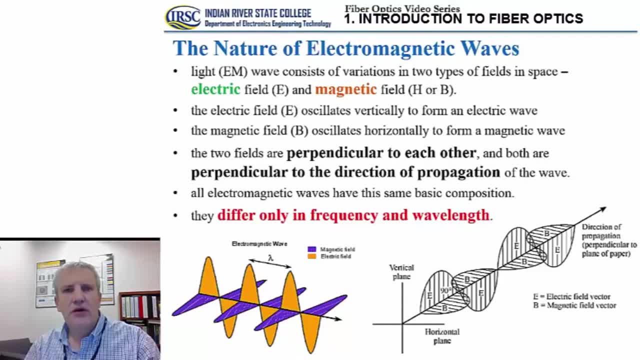 other. They're at right angle relative to each other. What we described here is so-called transverse wave. It turns out that there are different types of waves. There's so-called longitudinal waves and there's also so-called transverse waves. What do we mean by that? 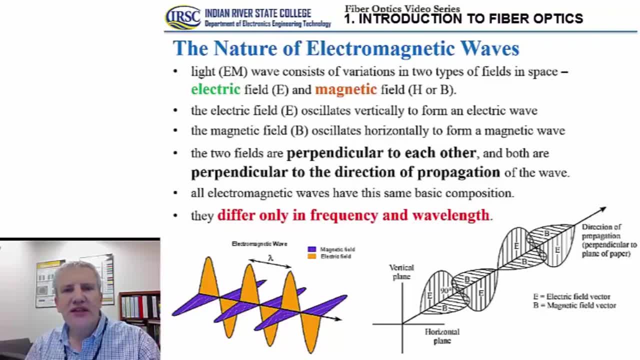 What do we mean by transverse wave? If you're looking at these two quantities that describe electromagnetic wave, namely electric field and magnetic field, they are perpendicular to each other and they're also perpendicular to the direction of the propagation. That's an important property of a so-called transverse wave. 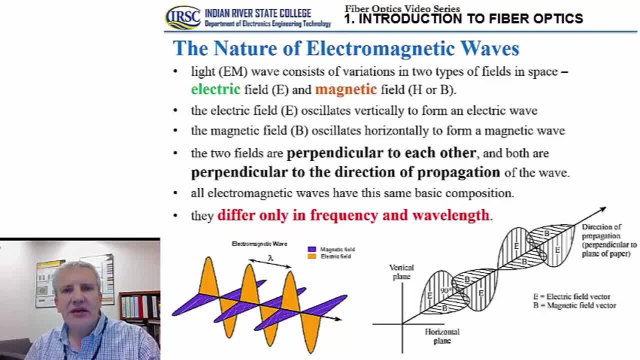 So the oscillation is basically taking place in a plane that is perpendicular to the direction of propagation. In the case of an electric field, we see that oscillation is perpendicular to the direction of propagation, So the oscillation is taking place in a vertical direction, right. 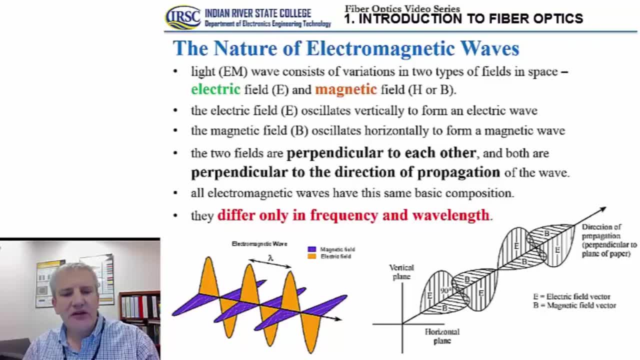 And then the oscillation of the magnetic field is taking place in a horizontal direction, and those two directions are perpendicular to the axis of the propagation. In the case of a longitudinal waves on the other side, you'll see that the disturbance of oscillation is going to be basically taking place along the direction of the propagation. 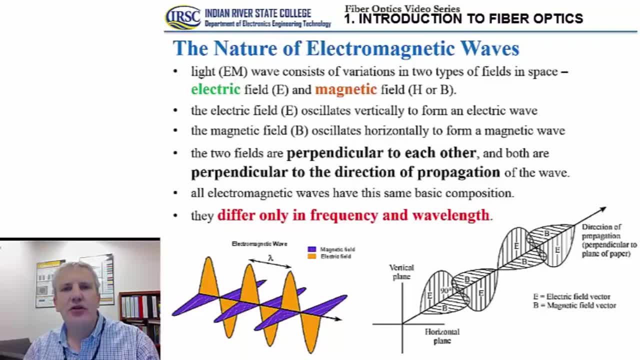 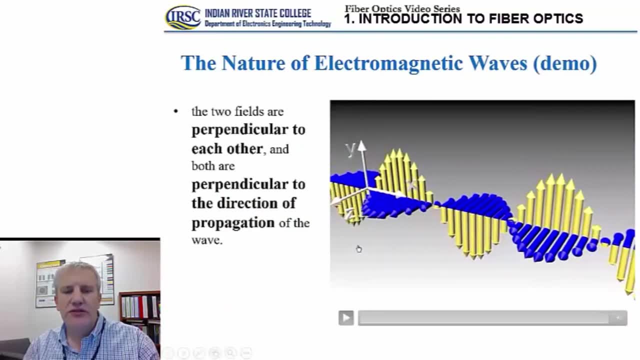 So that is a fundamental difference between the two. Thank you, Thank you, Thank you very much, Thank you very much, Thank you. Here we can see a short demo of an electromagnetic wave where yellow arrows represent the electric field and the blue arrows represent the magnetic field.